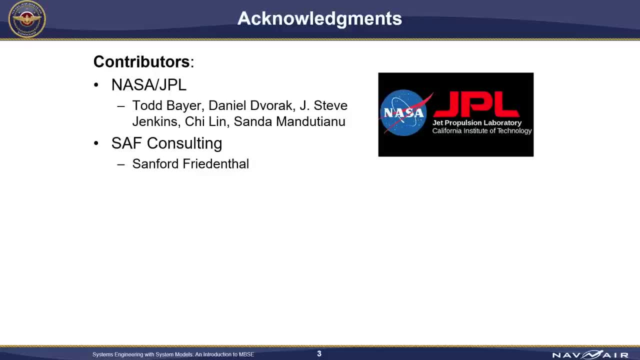 The NASA Jet Propulsion Laboratory, or the NASA Jet Propulsion Laboratory, is an international research institute in the United States. The NASA Jet Propulsion Laboratory in Pasadena, California, has been a pioneer in the transformation to model-based systems engineering. This training video was adapted from the first in a series of videos on model-based systems engineering produced by NASA JPL. 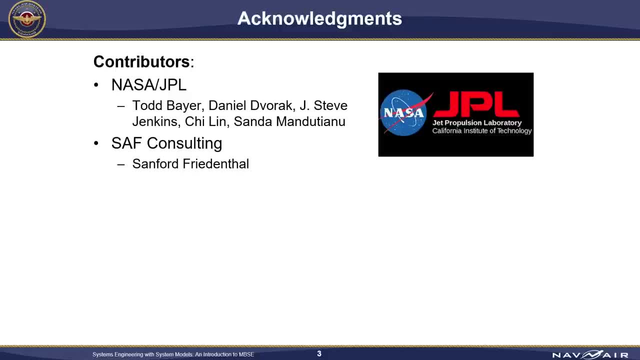 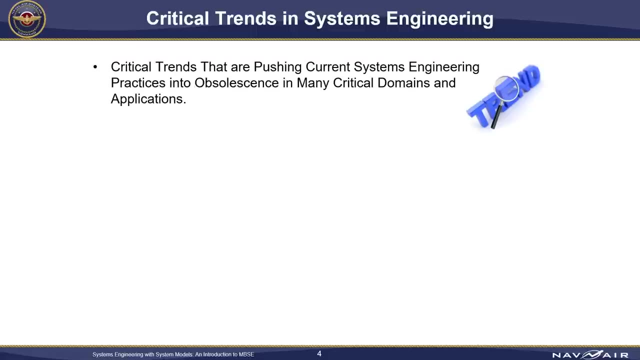 and NAVAIR would like to acknowledge the contributors to the original series. As you will see in this video, many of the references and case studies draw upon information from the Europa Study Systems Engineering Team and the JPL Modeling Early Adoption Program. Before we start examining the system model, let's take a look at some critical trends that are pushing current systems engineering practices. 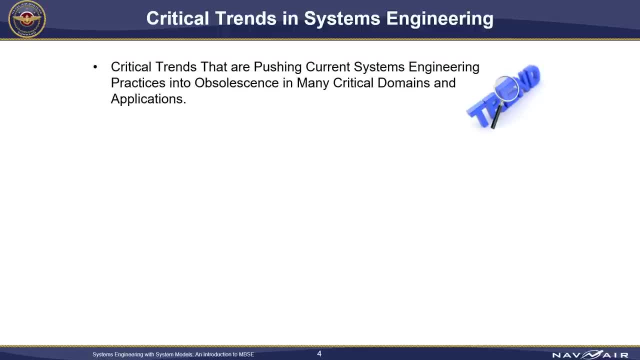 into obsolescence in many critical domains and applications. These trends are a result of the exponential increase in computing capability and storage, coupled with the exponential growth of network bandwidth. The first trend is that systems are becoming increasingly more complex, in both number of components and interconnectivity. 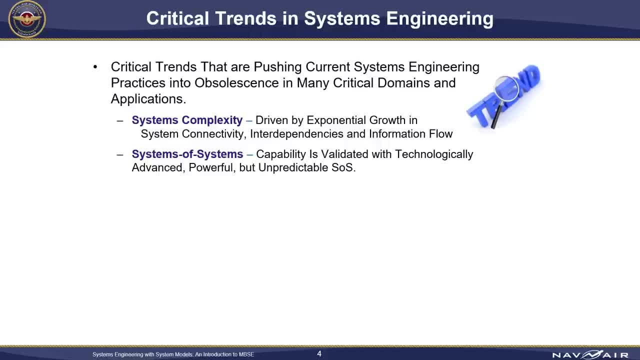 The second trend is our increasing societal day-to-day dependency on Technologically Advanced and Powerful, yet Unpredictable System of Systems. The third trend, which compounds the impact of the first two trends, is that a combination of customer expectations and evolving threats has greatly compressed the development timeline. 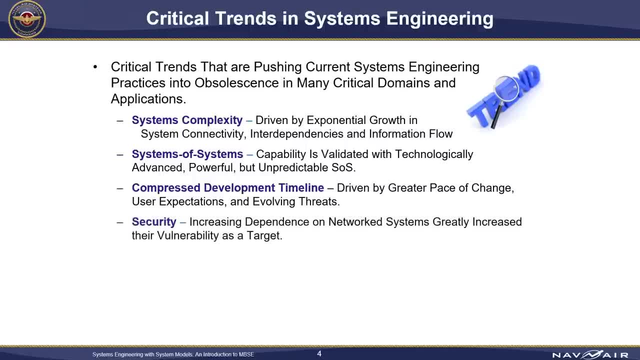 The fourth trend is related to security. Our increasing dependence on network systems has greatly increased the number of systems that are being developed. Our increasing dependence on network systems has greatly increased the number of systems that are being developed. Our increasing dependence on network systems has greatly increased the number of systems that are being developed. 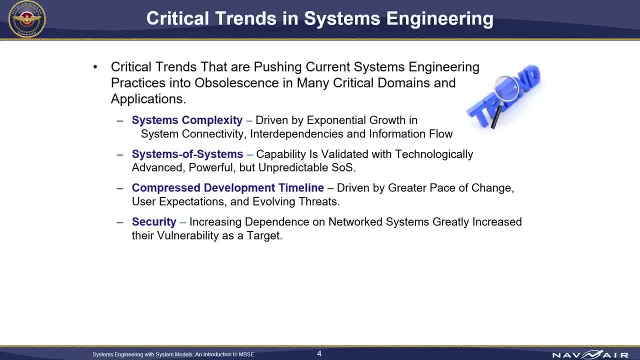 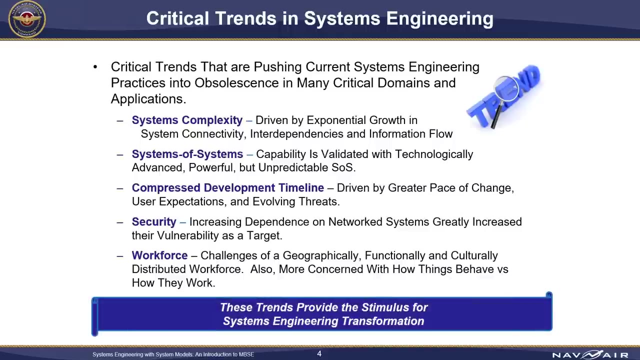 Our shrinking social security, where processes are being семpreded by the and by daggers, has brought about an increase in the intent of platformsного and language. We are seeing a rise in Financial perfomance. We are seeing a decrease in support for business development. 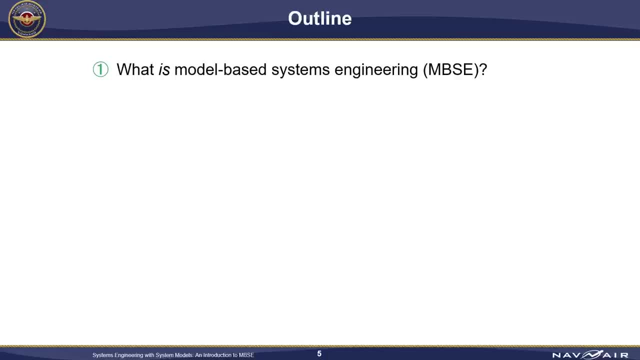 We are seeing a rise in performance. This module will begin with a couple of formal definitions of MBSC and will address the common question: what's the big idea behind MBSC? Then we will look at some problem areas in the current practice of systems engineering. 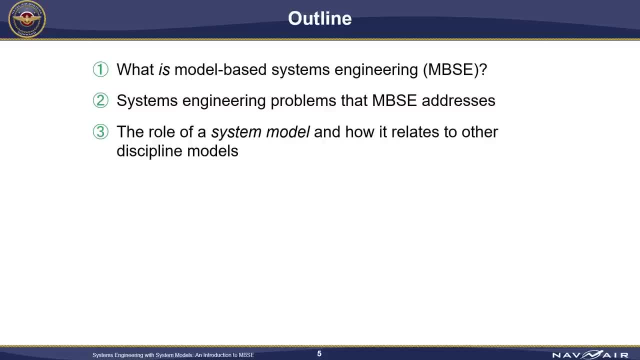 that MBSC helps address, and then look at the concept of a system model and the role that it plays, including its relation to other discipline models, such as mechanical and electrical models. Then, as a case study, we'll look at a project that is applying MBSC in the formulation. 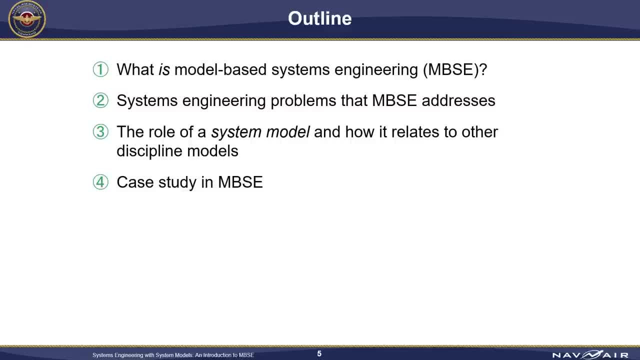 phase to see what systems engineering artifacts they have produced. That will be followed by a brief comparison of MBSC to more conventional SE, including observations from practitioners. We'll examine some of the management issues involved in moving to a more model-centric approach. Along the way, we'll look at some myths about MBSC in order to correct some misconceptions. 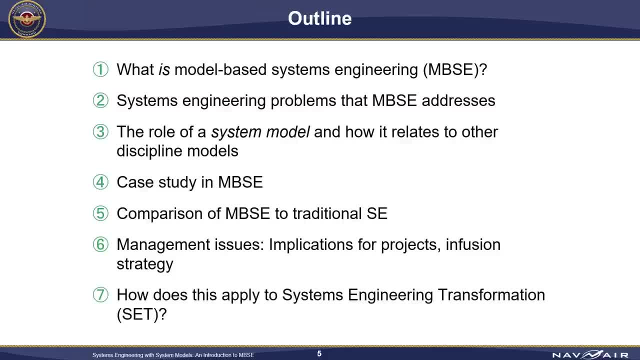 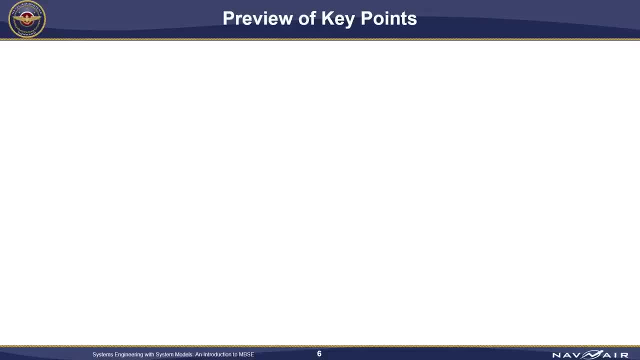 And finally, we will see how this applies to NAVAIR's Systems Engineering Transformation Initiative, also known as SET. Before we dive in, let's preview a few key points that will emerge in this module. First, it's worth keeping in mind that MBSC is fundamentally about doing good systems. 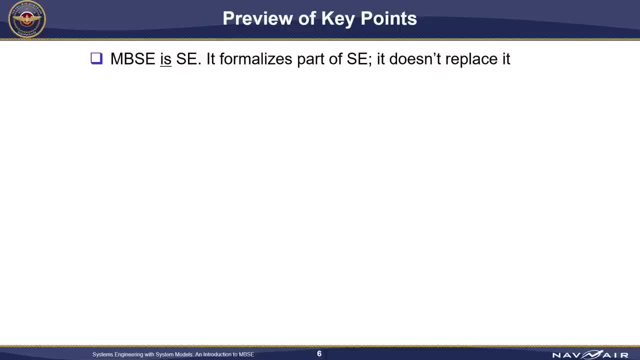 engineering. It's not a new religion and it doesn't replace systems engineering. Second projects that have applied MBSC are seeing better communication within teams as well as to stakeholders, better management of complex designs and improvement in the quality of products. 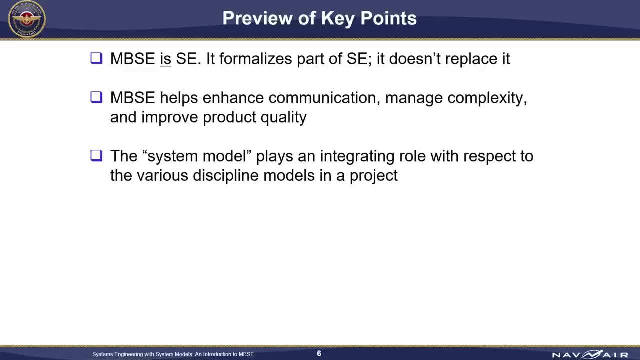 Third, we'll see that the so-called system model plays an important role as an integrator of design information in exchanging information with the various discipline models, such as mechanical and electrical models. Fourth, we'll see the ability of models to organize rich technical information and help. 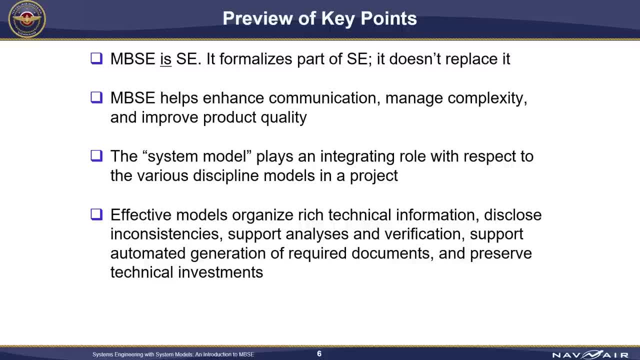 disclose inconsistencies, Well-organized models, support, analysis, verification and automated generation of required documents. Finally, infusion of MBSC principles and practices involves some learning curve and culture change, so it's best to plan for that. Okay, let's begin by addressing the obvious questions. 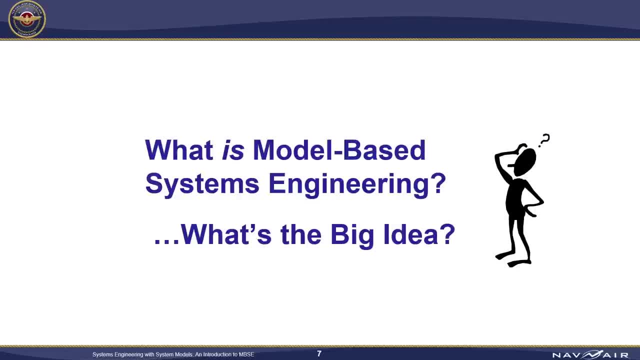 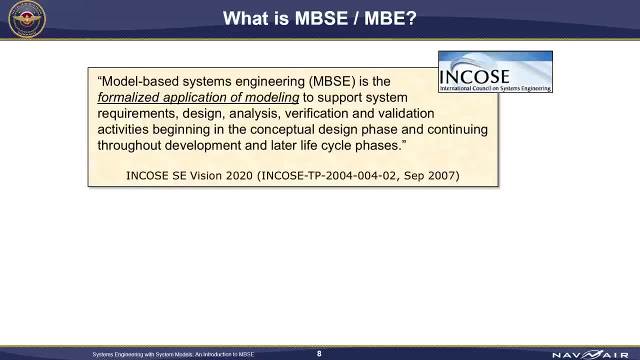 What is model-based systems engineering and what's the big idea? anyway, Let's start with a couple of definitions. According to NKOSI, the International Council on Systems Engineering, MBSC is the formalized application of modeling to support the engineering activities that systems engineers always engage. 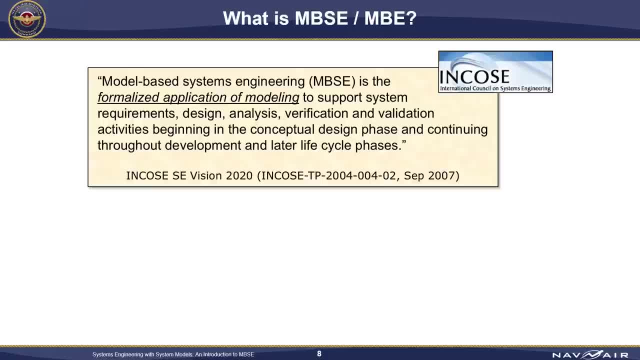 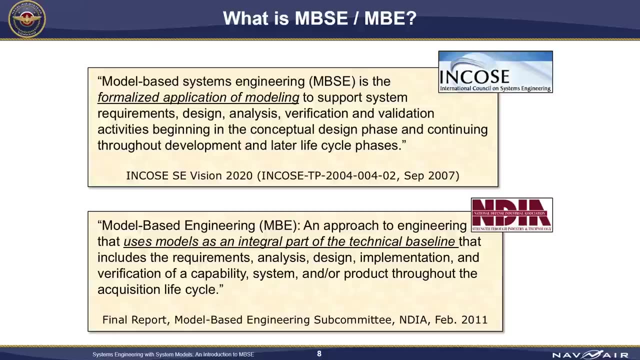 in, namely requirements, design, analysis, and verification and validation. The definition goes on to say that MBSC begins early in the project lifecycle and continues into later phases. Continuing on to the second definition, the National Defense Industrial Association emphasizes that model-based engineering uses models as an integral part of the technical baseline. 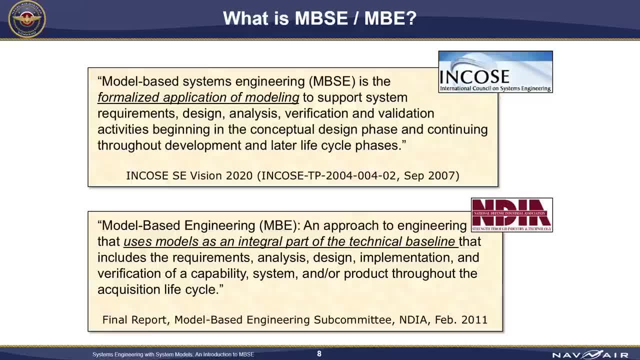 In short, both definitions emphasize the role of models in activities spanning the project lifecycle. In this module, we'll often use the phrase system model rather than just model to clarify that we're focusing on a system-level description. In this module, we'll often use the phrase system model rather than just model to clarify that we're focusing on a system-level description. 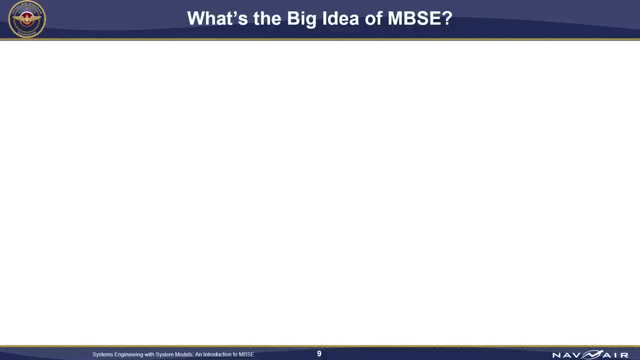 So what is the big idea of MBSC anyway? Well, the first idea is to add rigor and precision to our systems, engineering conversations and our work products. Miscommunication is one of the principal dangers in a project, whether it's due to errors of interpretation or errors of omission. 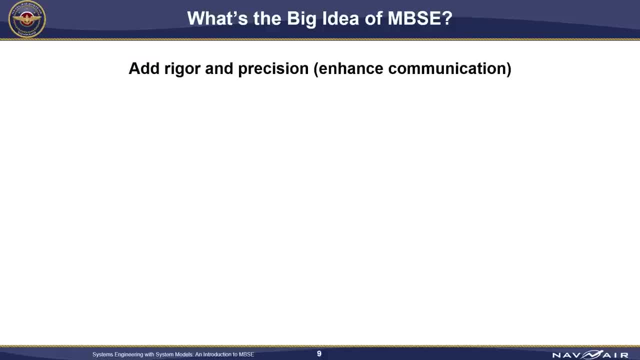 And that vulnerability to miscommunication increases as systems become more complex. The second idea is to help manage complexity in the increasing complexity of the project. The second idea is to help manage complexity in the increasing complexity of the project. The second idea is to help manage complexity in the increasing complexity of the project. 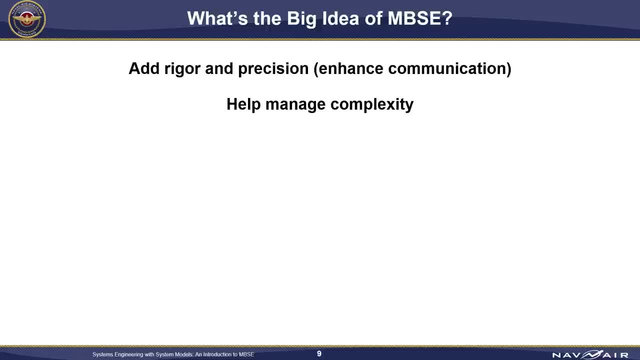 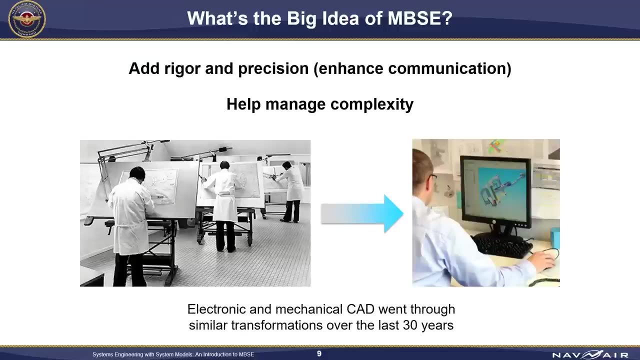 For a couple of reasons. We can either produce a very saudable model that won't have enough time to adapt to Our project is compensated for, But it is only possible to improve it ourselves. Transformation matters. Relax your head. is expected to be as real and important as it was for mechanical and electrical engineering. 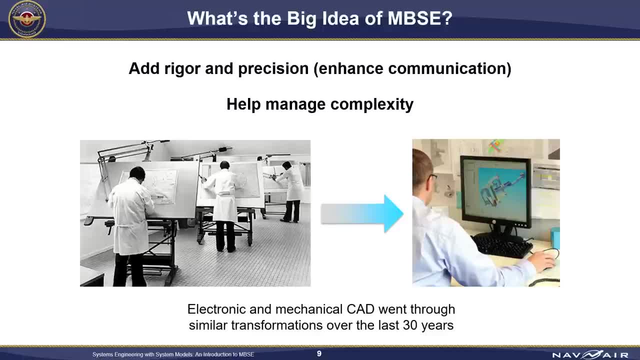 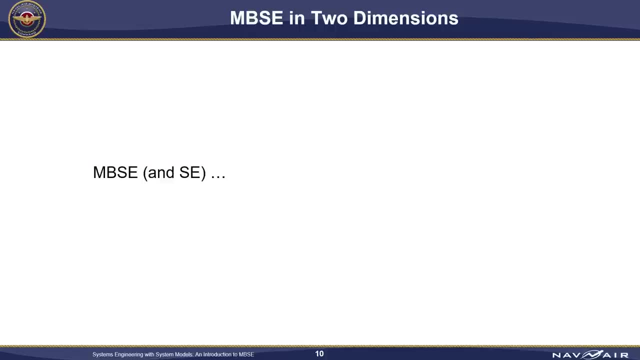 If you are wondering why systems engineering is late to this party, part of the answer is that there has been a lack of standards until recently, And another part is that systems engineering has been harder to formalize because of its breadth. This chart visually emphasizes two dimensions that MBSE shares with SE. 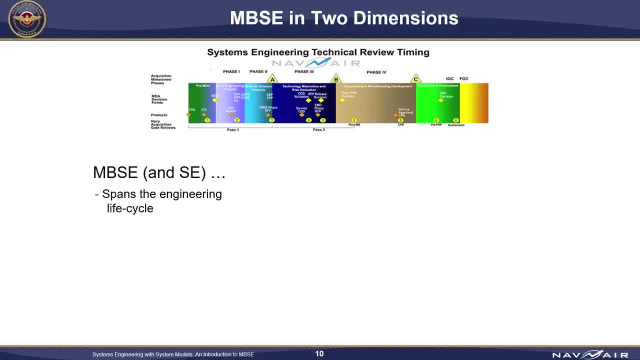 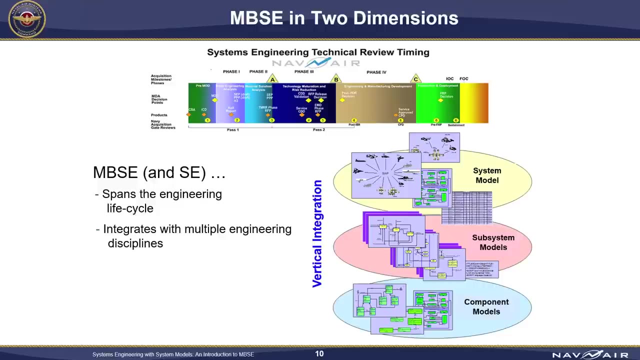 First, MBSE applies across the project lifecycle, from concept studies in pre-Milestone A to operations in FOC. That's the horizontal dimension, if you will. Second, MBSE focuses on a system-level description and of course that description must be consistent. 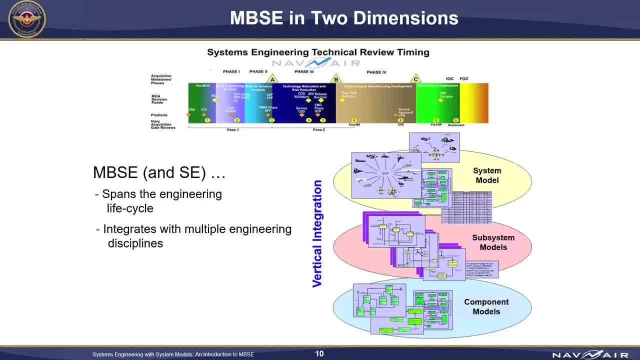 with the more detailed descriptions of subsystems and components. That's the vertical dimension. At the top of the vertical dimension is something called a system model, And that's what we'll explore next. Remember, the title of this module is Systems Engineering with System Models. 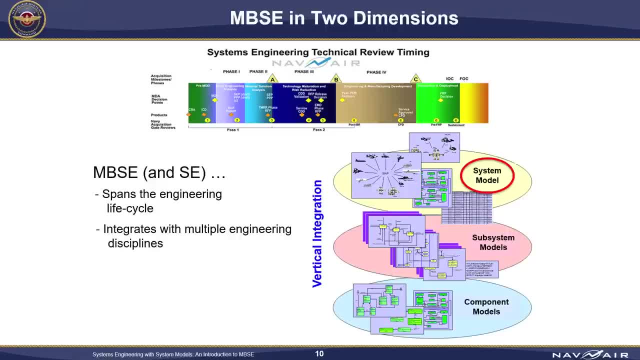 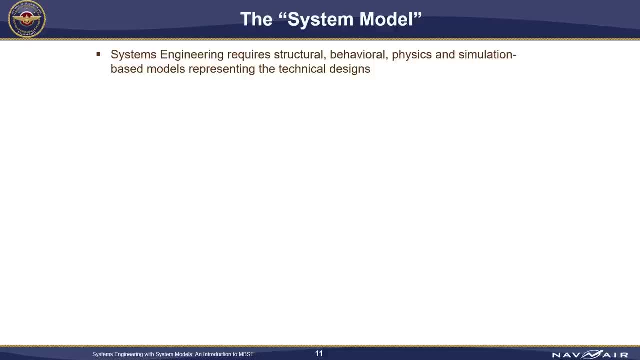 So, as we proceed, we'll be talking about the role that a system model plays in a project. Now, it has always been true that systems engineers work with models, including structural, behavioral physics and simulation-based models, to represent the technical designs. 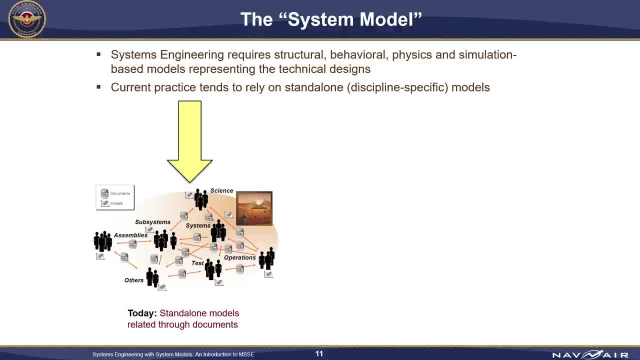 So what's different here? Well, one difference is that A system scientist tends to rely on stand-alone models. These are often discipline-specific models, such as mechanical, electrical, thermal, etc. that are loosely integrated and described in documents. Much of the formal communication among the different engineering teams takes place through a variety of documents. 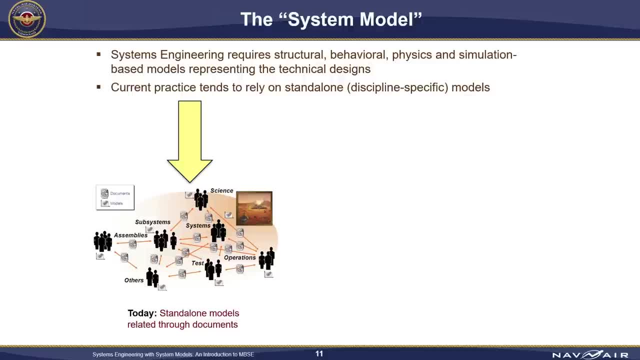 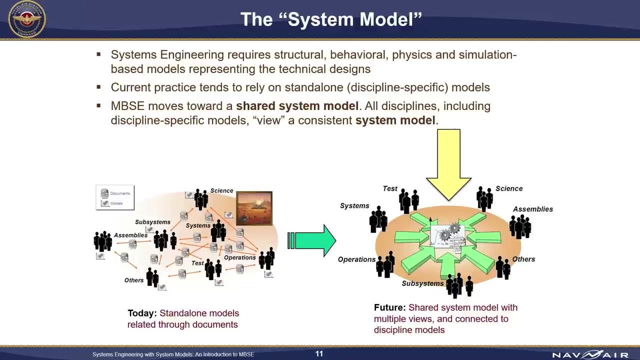 that include human-readable text, diagrams and spreadsheets. The challenges in this traditional approach are: one, ensuring consistency among all the documented models, especially as the design evolves, and two, just getting a system-level understanding of the technical baseline. What's different in MBSE is the move toward a shared system model. 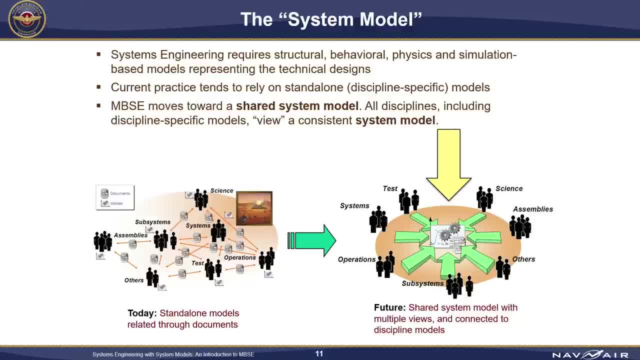 There will be more about the system model in a few minutes, but it's worth noting here that the system model is both human-readable and computer-readable and therefore more easily checked in an automated way for completeness and consistency. The system model becomes a basis of communication at a system level. 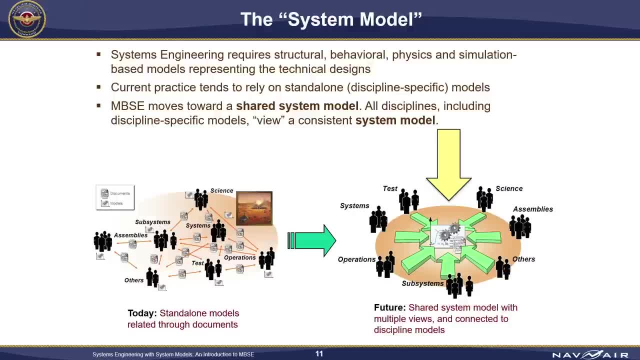 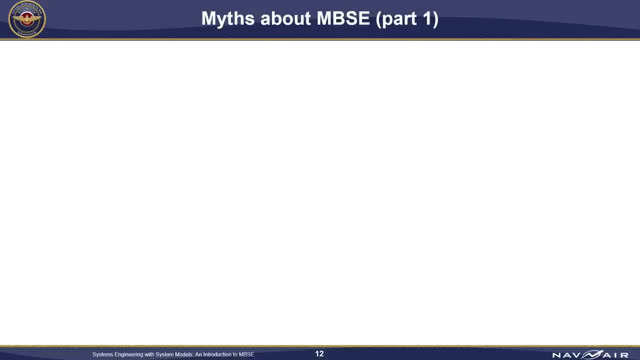 not only for humans to understand the evolving baseline, but also for integrating information across the various discipline-specific models. Now, before we leave this section, it is useful to note that there are some misconceptions about MBSE, So let's take a look at three of them. 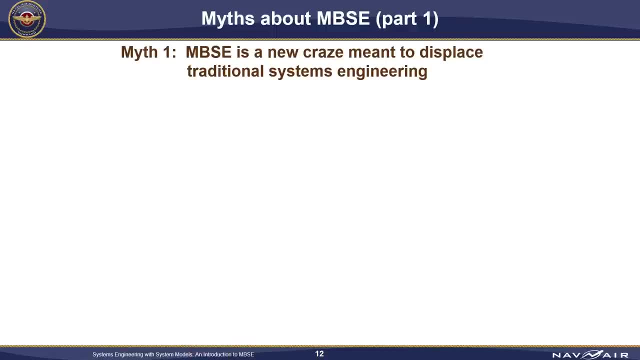 The first myth is that MBSE is some kind of new craze- or new religion, if you will, that aims to displace traditional systems engineering. and the short answer is no. MBSE doesn't displace traditional SE. What it does is transform the practice of systems engineering. 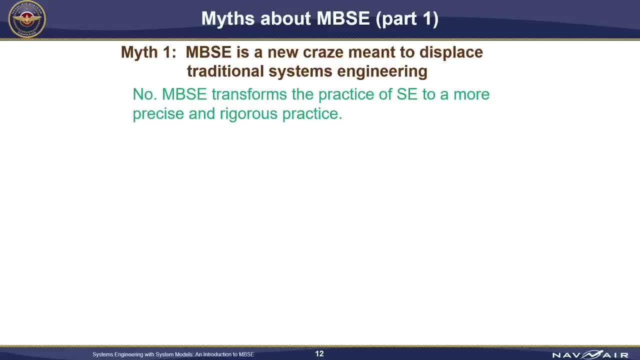 to a more precise and rigorous practice. Another myth is that MBSE is an additional SE activity on top of what systems engineers already do. The reality is that MBSE is pure technique. It is technique for doing systems engineering, just as electrical CAD is a technique for doing electrical engineering. 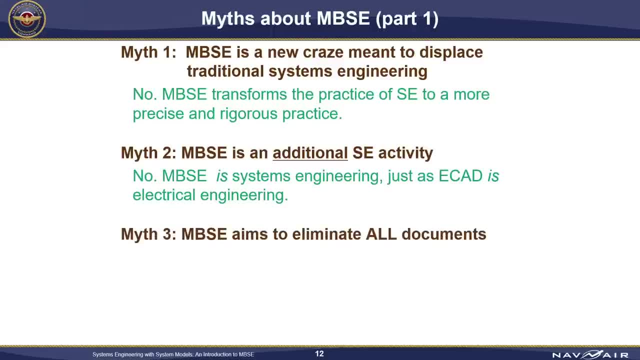 It's not an additional activity. A third myth is that MBSE aims to eliminate all documents, and that's understandable, given that MBSE is often described as moving from a document-centric approach to a model-centric approach. However, some documents may still be important. 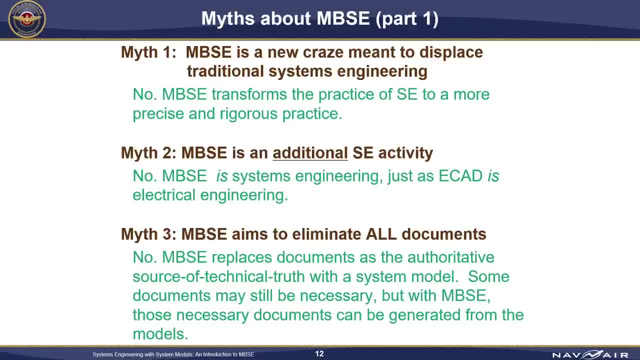 and even desirable. A well-structured document containing a thoughtful narrative can convey important facts and analyses in a way that directly addresses stakeholder concerns. What's possible now with MBSE is to keep required documents mutually consistent and up-to-date by generating documents from an authoritative integrated system model. 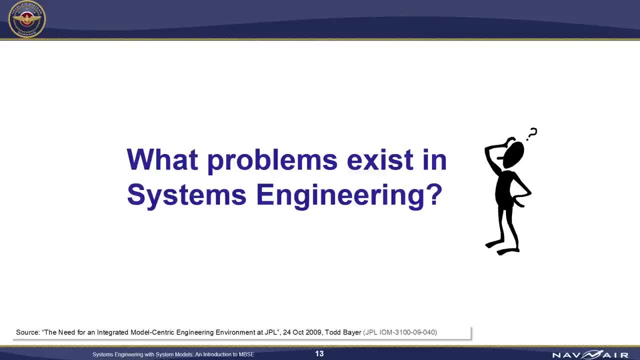 Moving on. let's look at some of the problems that have been identified in the practice of systems engineering, And later we'll see how MBSE addresses these problems. What you'll see in the next few slides came from a 2009 study at NASA JPL. 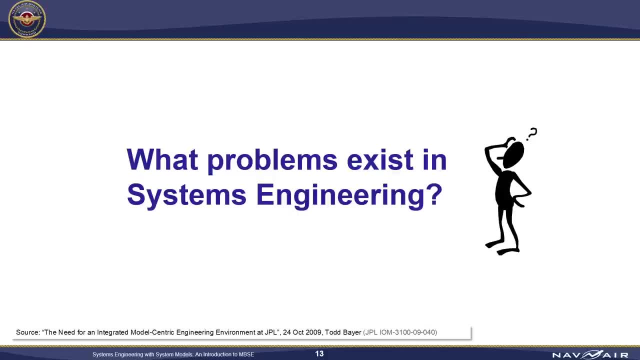 that examined several reports about systems engineering in order to understand the problem areas and establish some concrete goals for what to fix. The study was conducted by JPL's Initiative on Integrated Model-Centric Engineering and five themes emerged, Although this was a NASA study based on space. 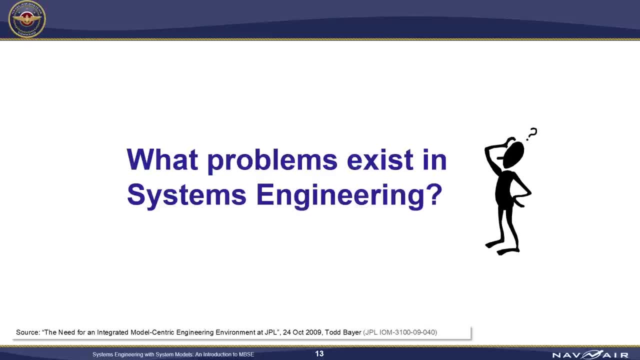 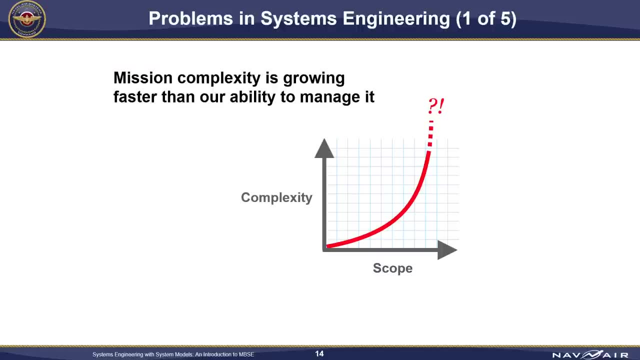 you will see very close alignment to what is happening with naval aviation. The first problem is that mission complexity is growing faster than our ability to manage it. Missions have become increasingly ambitious, evolving from fly-by reconnaissance to orbital studies to in-situ exploration. 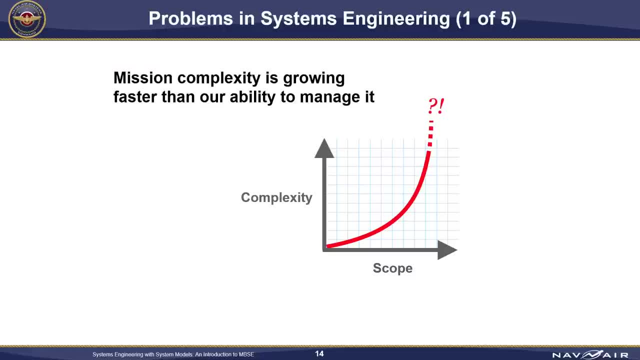 and that has been enabled by ever-increasing space-borne processing capability, with more and more flight system functionality implemented in software. Unfortunately, single viewpoint natural language specifications are inadequate to capture and expose these system-level interactions and characteristics, increasing the risk of unexpected system behaviors. 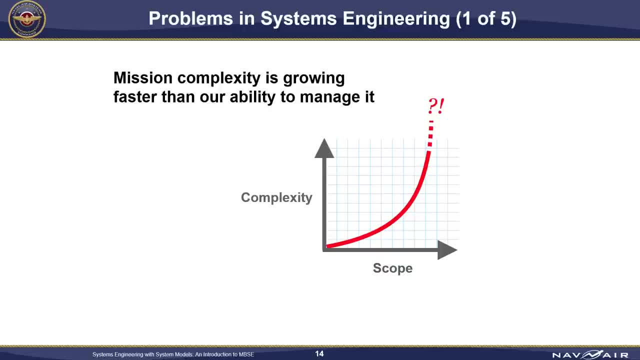 At the same time, the potential range of behaviors has become so large that it is impractical to fully test it. Problems can no longer be reliably exposed by testing. The result of this situation is that inadequately specified and incompletely tested system-level interactions 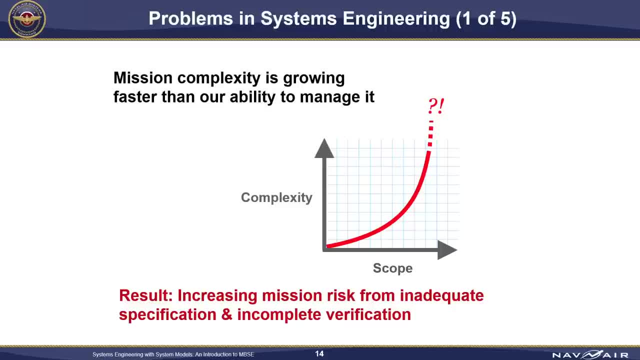 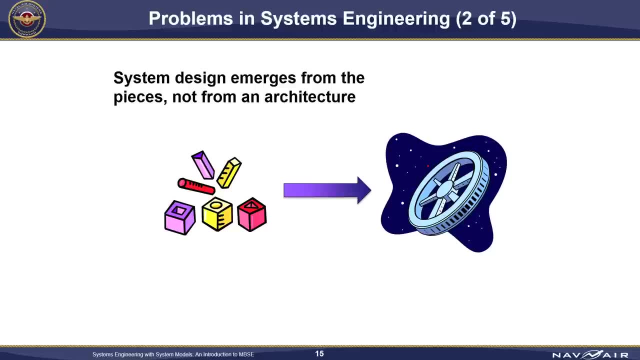 are a major and growing risk factor for our missions. The next problem is that system design often emerges from the pieces rather than from an architecture. Architectural principles are seldom articulated or used to drive the design, and that allows poorly understood or flawed requirements and assumptions. 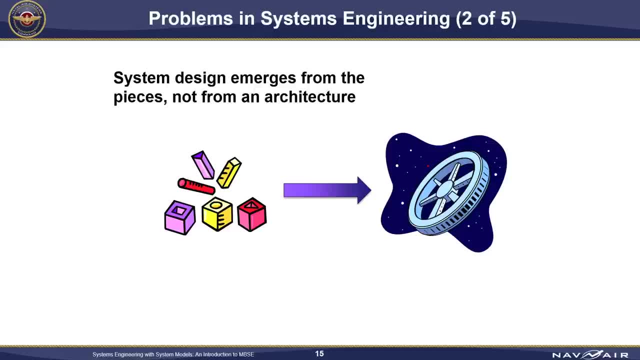 to persist, resulting in weakened designs In general. weak architecture can be a challenge and can lead to unmanageable interactions, stove-piped analyses, brittle fault protection, untestable aspects of design and late discovery of design defects, such as unexpected behaviors and unmet requirements. 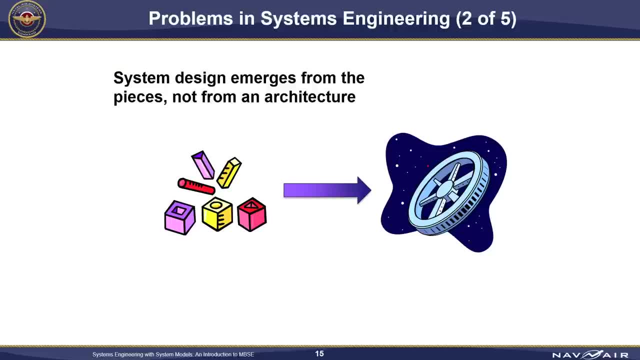 Also, with so much of system behaviors managed by software, it's crucial that systems engineers communicate effectively with software engineers, but textual representations are often ambiguous or incomplete. The result of all these issues is that we end up with systems that are brittle, difficult to test and hard to operate. 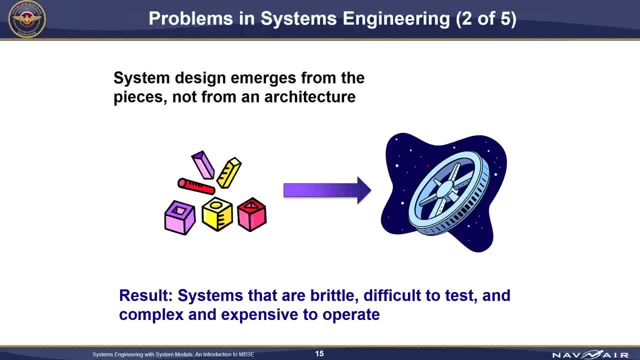 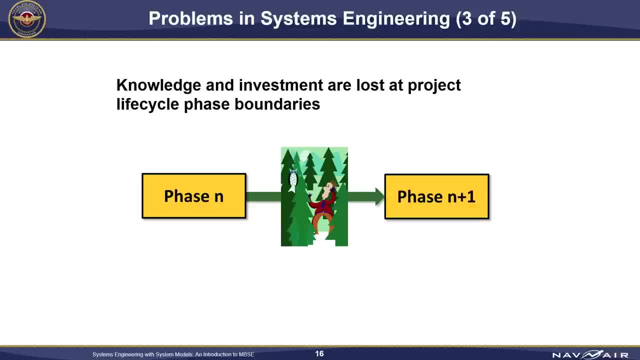 In fact, we end up with systems whose behavior must be discovered, often in flight. The third problem is that knowledge and investment are lost at project lifecycle boundaries. For example, models used during the formulation phase of a project are abandoned and new ones created when the implementation phase begins. 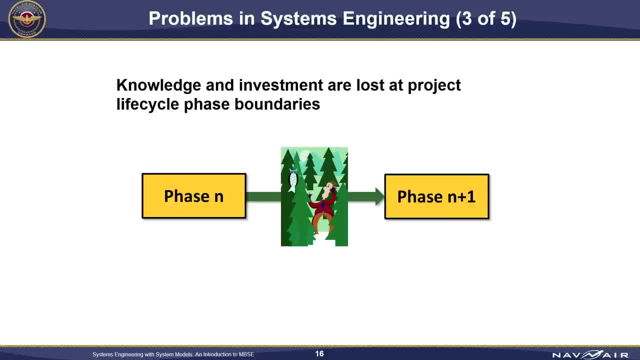 Many examples exist, including trade models, cost models, power, telecom and data transport models. Essential attributes of design are not captured consistently in a readily accessible manner, For example, architectural principles, trade study assumptions and rationale system. design rationale and narrative are only partially captured, at best. 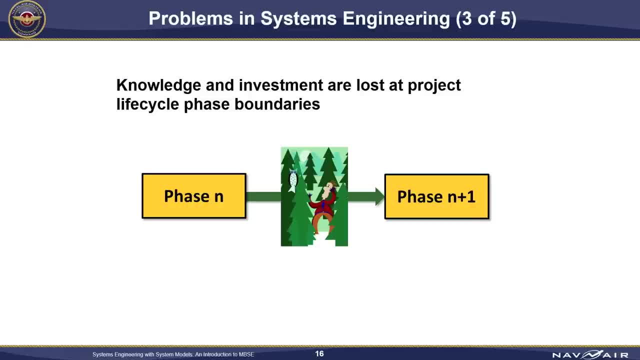 and are seldom readily accessible. Training of engineers joining a project takes longer than necessary. In moving from pre-Milestone A to FOC, there is significant team expansion and turnover. Training people who were not around for the previous phases is currently heavily dependent on getting key documents from 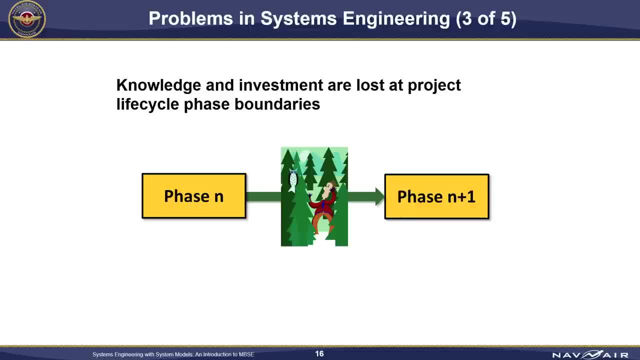 and having lengthy conversations with key people Because the system design is poorly captured. this essentially ensures that new team members will be discovering attributes of the design for years. The net result of all this is that the risk of late discovery of design problems increases developmental timeline and cost. 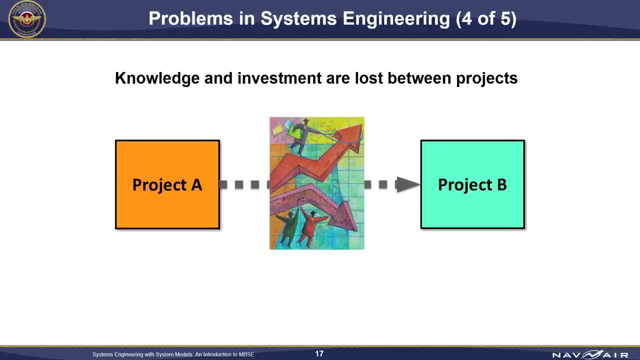 The fourth problem is that knowledge and investment are lost between projects. Since system architectures and designs are not well captured, reusing them on subsequent projects is difficult and seldom happens, except where the project team itself is inherited by the next project. There is currently no formal way to document and integrate 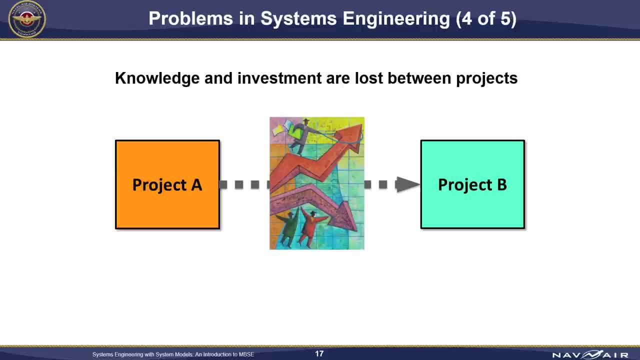 the broad experience of knowledge of engineers across a project, to train new systems engineers who will need to absorb this broad knowledge quickly and deeply, and to make this available as a legacy to future projects in a manner that's easily dissected and reapplied to new circumstances. 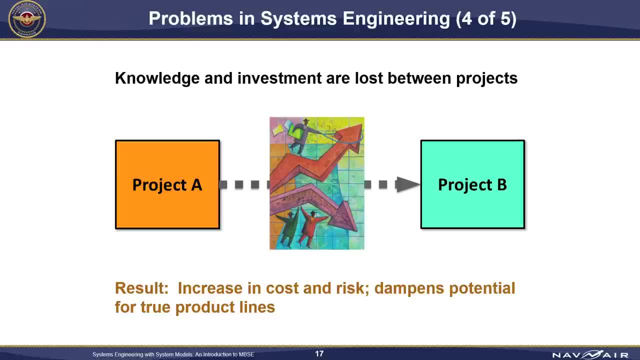 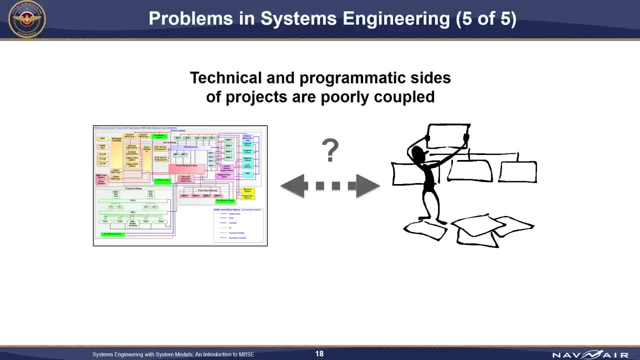 The net result is an increase in cost and risk compared to what could have been. Also, this problem reduces the potential for true product lines. The last problem area is that the technical side of a project is poorly coupled to the programmatic side. 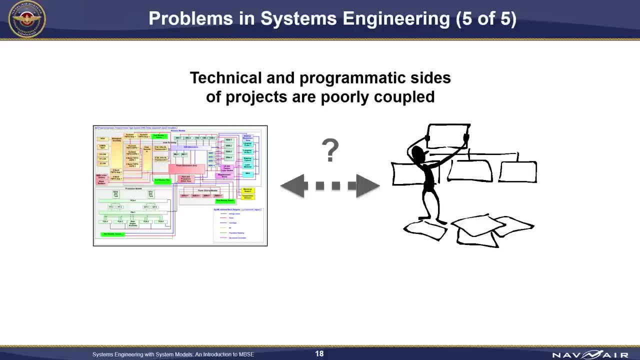 The cost schedule, scope, investment and risk implications of a given set of requirements, science, objectives, components and functions are very difficult to determine. Very little coupling exists between the performance side, which is science, requirements, components and functions, and the implementation side. 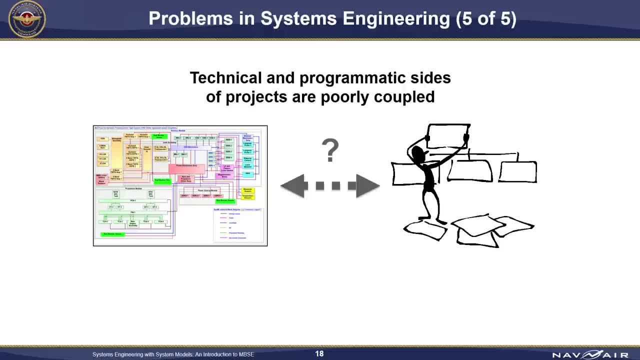 which consists of implementation, investments and risks. Project models rarely include mitigations or backup options for technical implementation risks. It is difficult to transfer information between tools and different discipline types. Trade studies seldom fully incorporate programmatic considerations, But it's important that systems engineers be knowledgeable about programmatic realities. 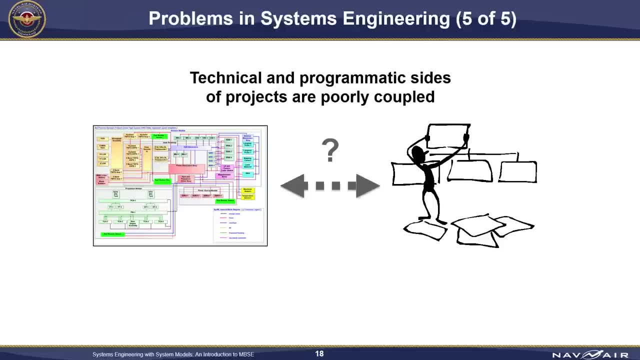 and the impact of engineering decisions on programmatics. However, existing tools don't support such an integrated view. The net result is that this poor coupling hampers effective decision-making on both sides- technical and programmatic- and that increases development risk. 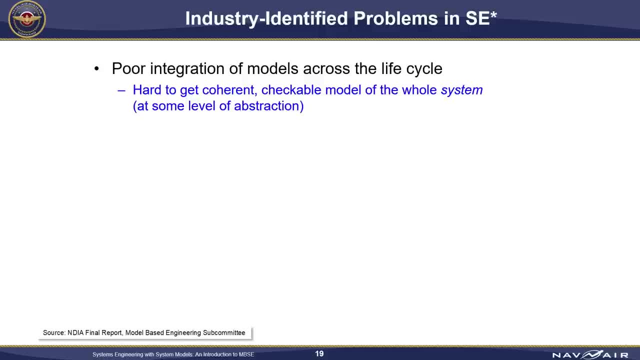 Before we leave this topic, it's worth noting that the National Defense Industrial Association noted similar problems with systems engineering. For example, they too saw poor integration of models across the lifecycle, making it hard to get a coherent and checkable model of the whole system. 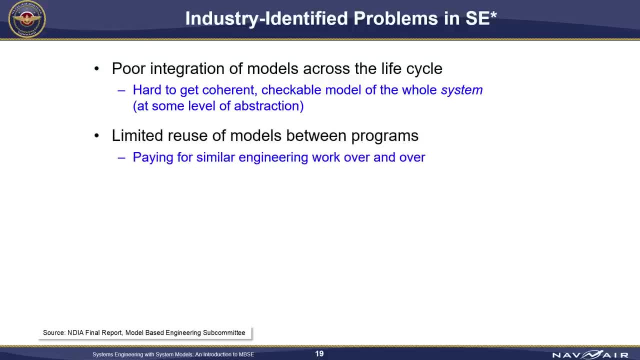 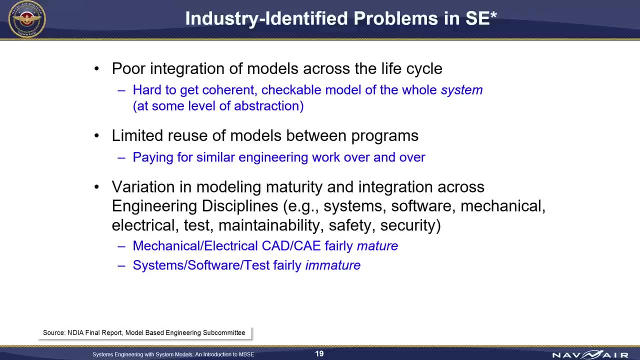 at some level of abstraction. They also noted the limited reuse of models between programs, which meant that sponsors end up paying for the similar engineering work over and over. They also noted that modeling maturity and integration varied across different engineering disciplines, with mechanical and electrical being fairly mature. 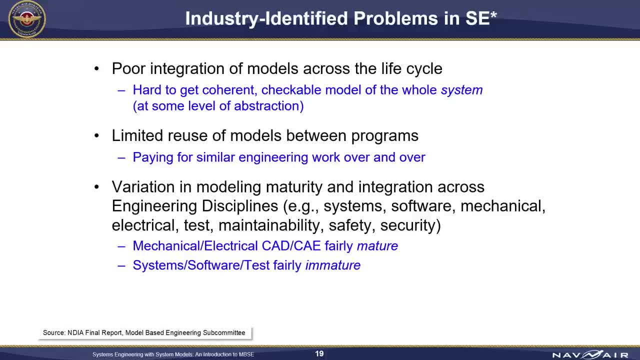 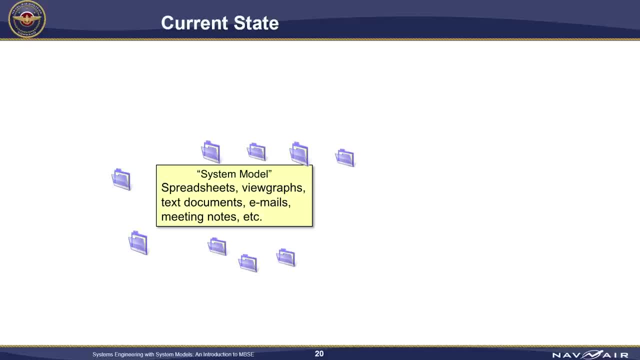 whereas systems and software and tests were fairly immature. So let's wrap up this topic by looking at where many organizations are today and where we would like to be. In sketching this picture, we're going to oversimplify a bit to make a point. 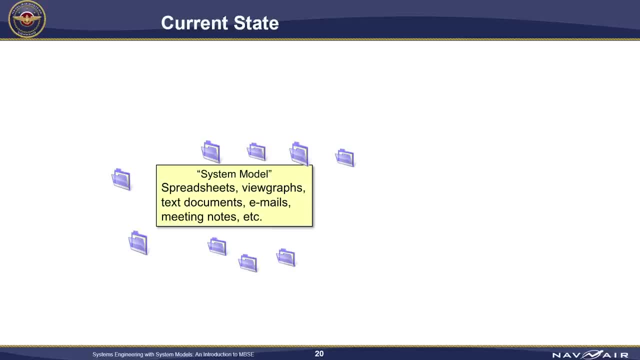 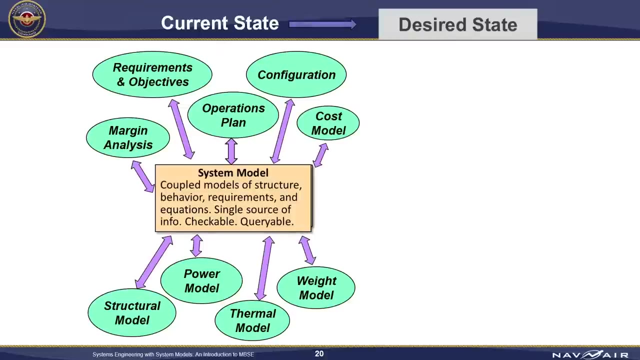 In the current state, most organizations have a system model of sorts consisting of spreadsheets and view graphs and text documents and emails and meeting notes, And this system model is loosely coupled to other models and plans through documents. Ideally, this rather weak notion of a system model. 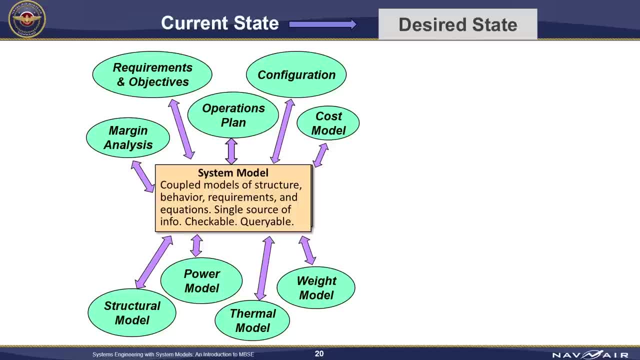 will give way to a much stronger notion in which models of structure and behavior and requirements and equations are coupled so that the relations among these elements are explicit. Such a model would serve as a single source of information at a system level and would be checkable for various types of consistency and completeness. 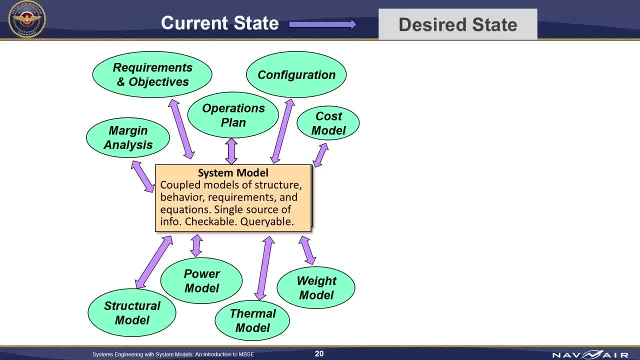 and queryable in the sense that the model can help answer certain types of questions. Looking to the future, we see a desired state where several things are different: Architecture and design captured in a formalized system. model Design reviews consist largely of model inspection and validation. 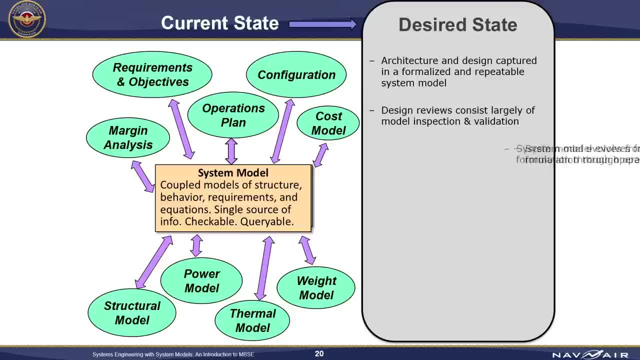 and examining key analyses that the model supports. The system model evolves across the lifecycle from formulation through operations. System test activities focus a lot of attention on model validation. given the importance of an integrated system, model Models and modeling tools are integrated across the lifecycle. 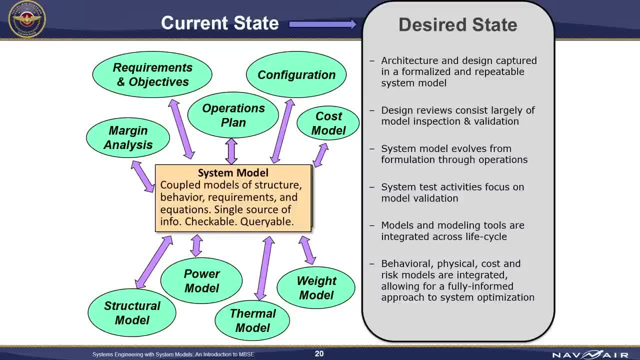 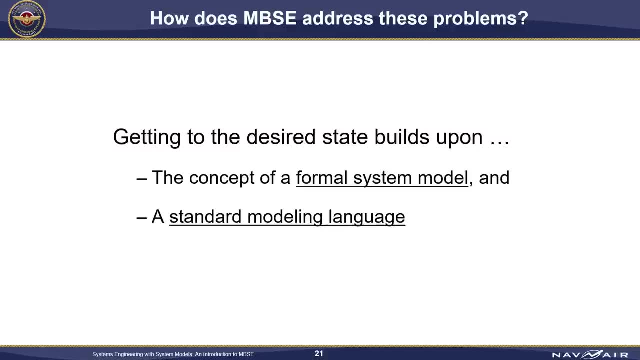 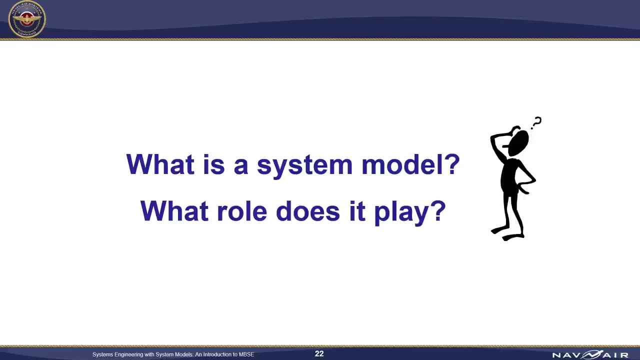 And finally, different types of models are integrated, allowing for a more fully informed approach to optimization. So that's the desired state. Getting to the desired state builds upon the concept of a formal system model and a standard modeling language. So let's now examine a couple of obvious questions. 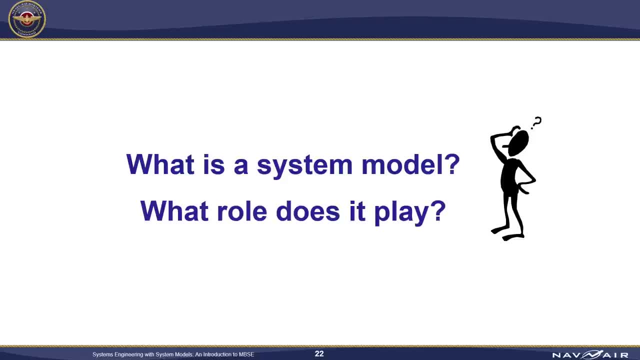 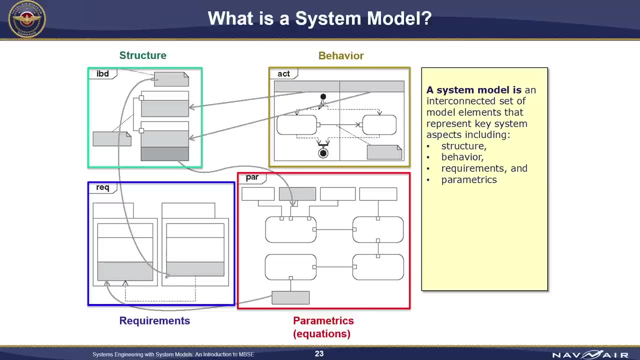 What is a system model and what role does it play? The answers in this section are fairly simple. We'll see more detail about a system model later in the case study. A system model represents four aspects of system design: structure, behavior, requirements and parametrics. 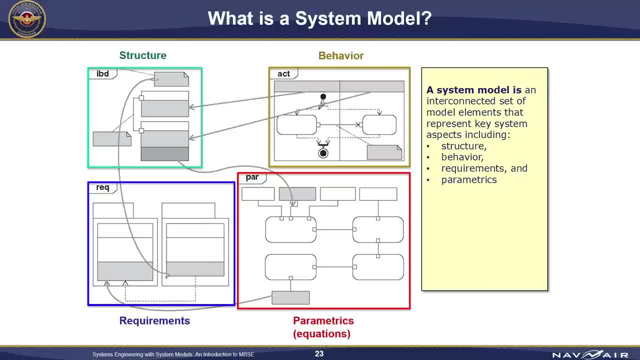 Understand, of course, that these aspects of system design are not new Systems engineers have always dealt with these aspects. What's different here is that these aspects are captured in a single model and in a way that they are coupled. For example, requirements are coupled. 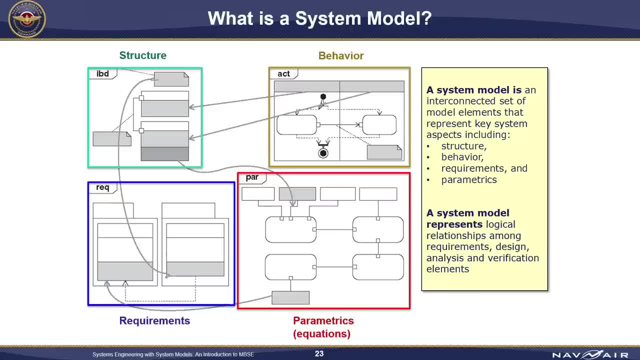 to elements of the design that they specify, such as components and interfaces and functions. Likewise, equations used to analyze parts of the design are coupled to the parameters that characterize components and behaviors or that are specified in requirements. We'll see more about this coupling shortly. 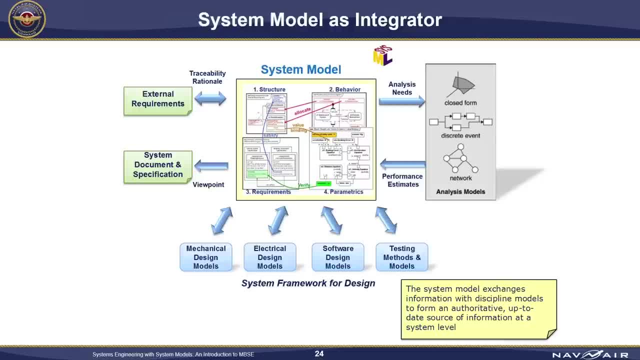 The next idea to keep in mind is that a system model plays an integrating role in analysis and design, and verification and operations. As this diagram shows, the system model receives information from other discipline models and it supplies information to other discipline models, For example, the mass properties of an aircraft. 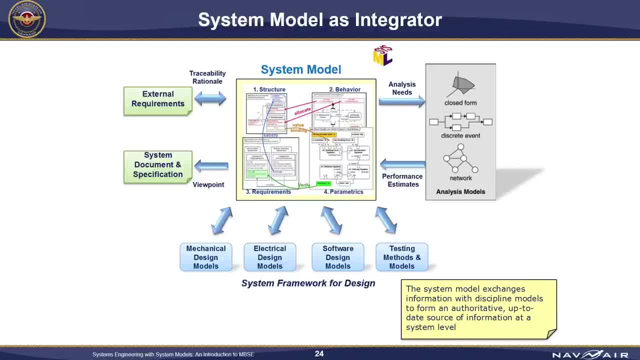 that come from a mechanical CAD model are kept up to date in the system model and supplied to other discipline models that need such information, such as attitude control analyses. Similarly, performance requirements held in the system model are supplied to appropriate analyses to check if the design satisfies the requirements. 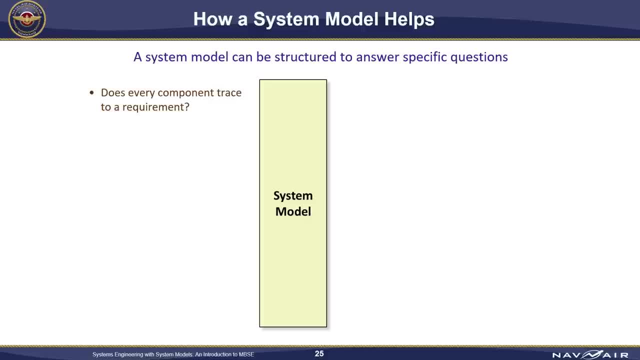 Let's look at how a system model helps. A system model can be structured to answer specific questions. For example, does every component trace to a requirement? The answer might be yes. Have both sides of every interface been specified? A script can check the system model. 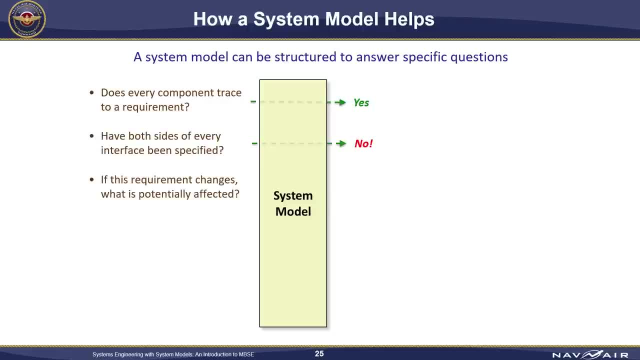 and determine if it is true or not. If this requirement changes, what is potentially affected? In principle, you can get a list of functions, components, interfaces and requirements that are affected. What is the weight of the hydraulic system, Again, with a properly structured system model. 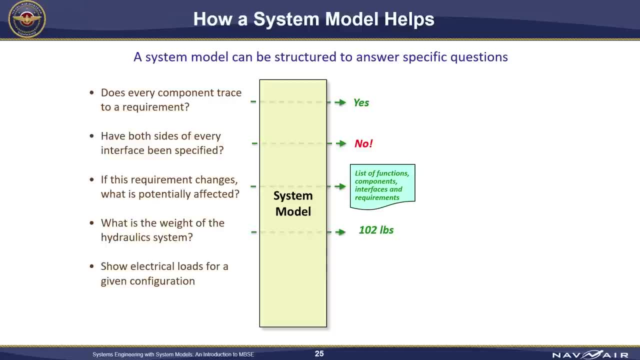 that can be answered with an analysis script. Show electrical loads for a given configuration. You could get an electrical loads profile for that kind of scenario. We'll see an example of that later in this module. What is the weight roll-up? You could get a master equipment list with the weight roll-up. 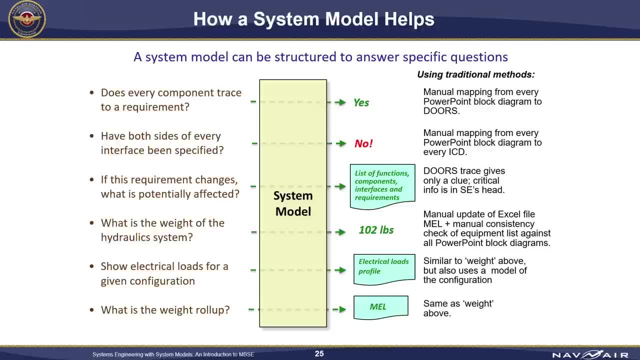 All of these approaches are done using traditional methods. There is a lot of manual mapping and in some cases the information is in a systems engineer's head. It is not explicit in the tool or in any of the statements. This emphasizes that a system model 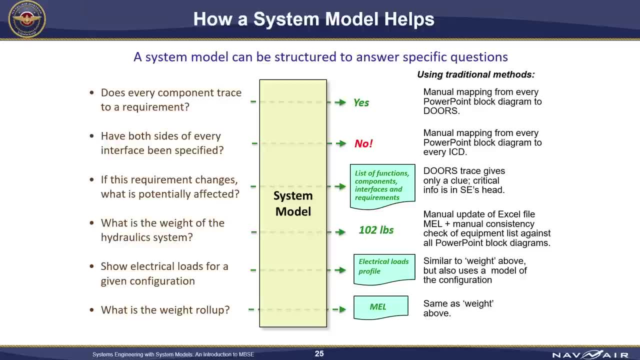 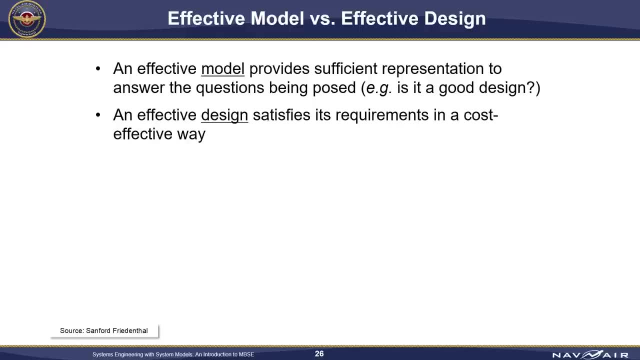 can help answer some of these questions automatically. It's useful to make a distinction between an effective model and an effective design. A model is effective if it can help answer the questions being posed. We model for a purpose, and that purpose includes answering questions such as: 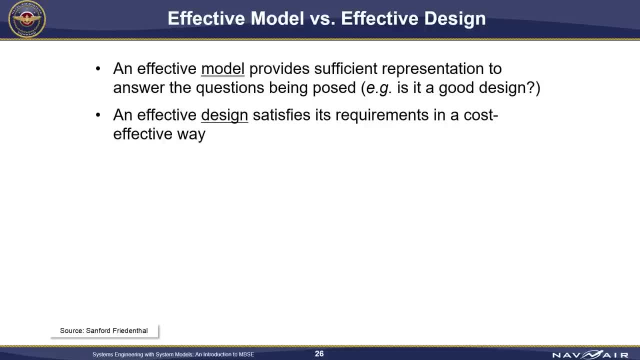 Does the design satisfy the requirements? Does the design have adequate margin in all operational scenarios? Will fault management properly handle a given failure? A simple example to make the distinction is a CAD model of a chair. It is certainly a high-quality representation of the chair geometry. 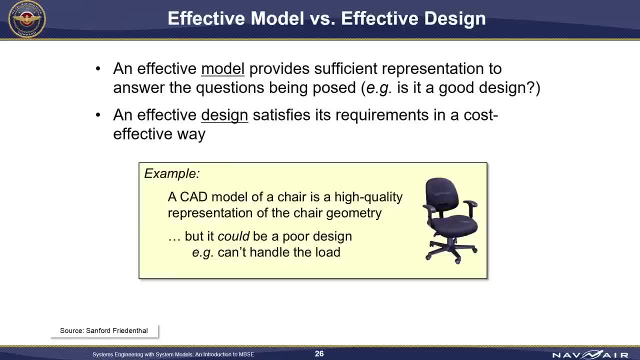 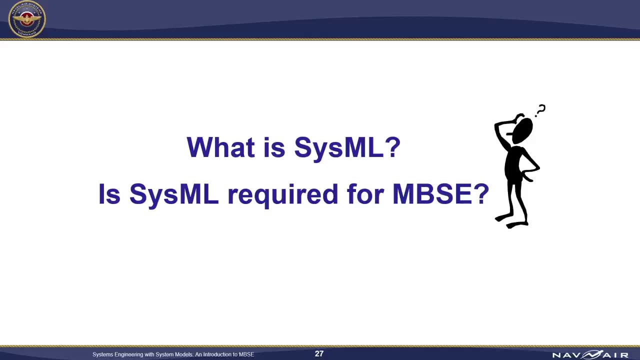 but it might be a poor design if it can't handle the required load. An effective model will tell us. The bottom line here is that a model is particularly helpful if it can show a flawed design to be flawed. Let's examine the question of 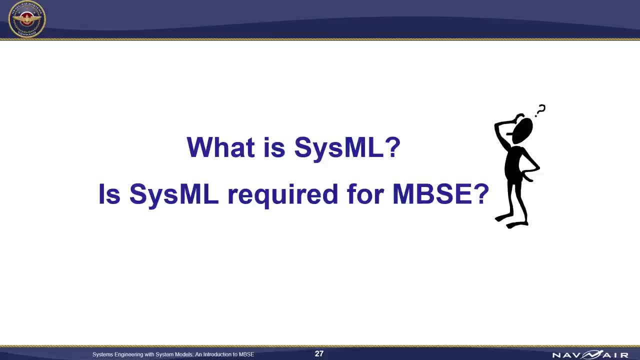 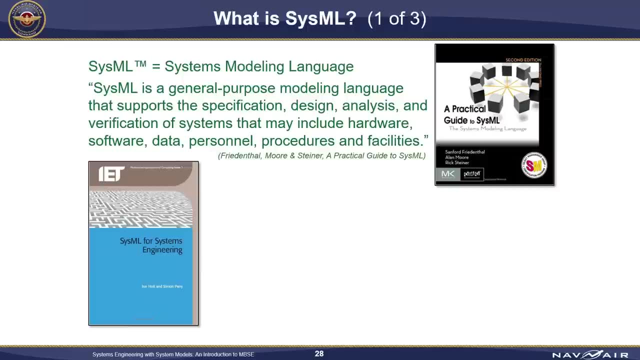 What is SysML And is SysML required for MBSE? SysML stands for Systems Modeling Language, which is a general-purpose modeling language designed to support systems engineers in what they do, namely specification, design, analysis and verification of systems. 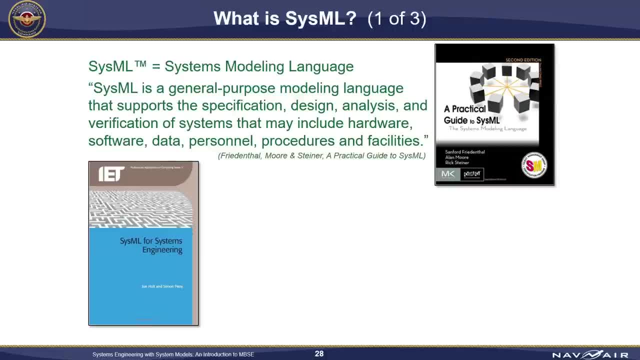 And the kinds of systems that SysML is designed for include hardware, software, data, personnel, procedures and facilities. It is very much a general-purpose modeling language. It's important to know that SysML is a visual modeling language that has several types of diagrams. 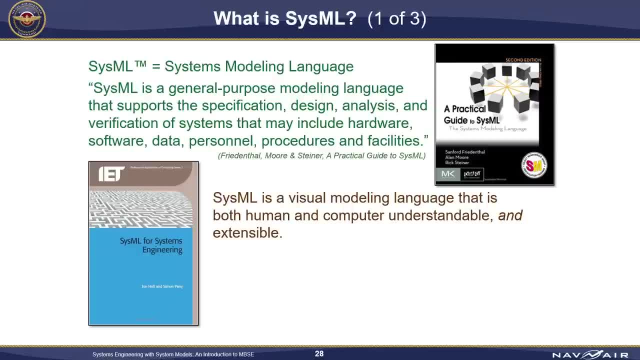 However, unlike diagrams that you might draw in PowerPoint, the information in a SysML diagram exists in a database, which means that it can be processed in various ways by computer programs. We'll say more about that later. The other important thing to know: 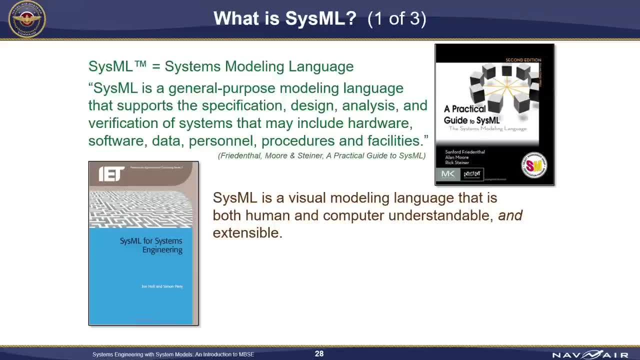 is that the language is extensible. For example, the language has a very general modeling element called a block, But that can be extended or specialized, if you will, to be a hardware component And that may be further specialized to be a flight hardware component. 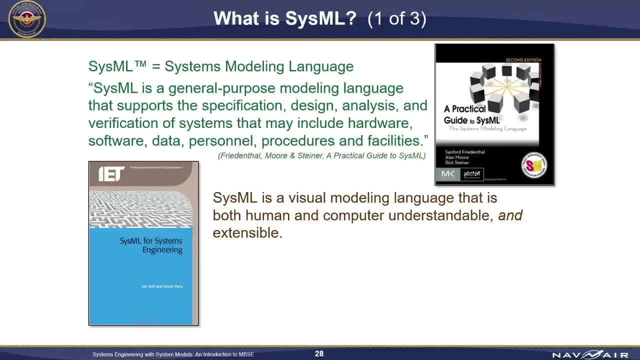 which therefore has mass properties And that might be further specialized to be an EGI, which has additional properties. Finally, this last quote about SysML being an industry-standard language designed to support modern systems engineering, simply points out that SysML. 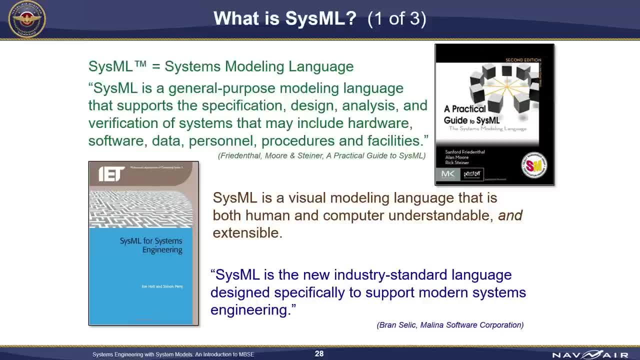 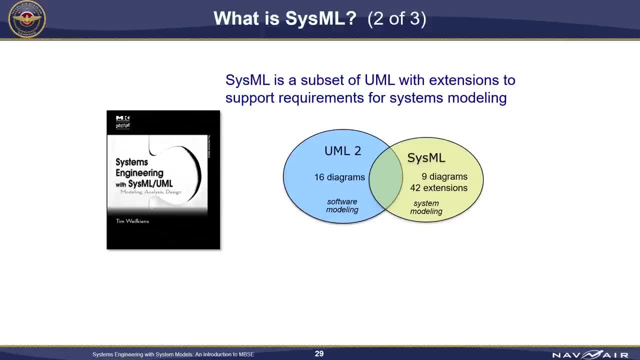 is an industry standard, not a proprietary standard, And in fact, it is currently supported by several commercial tools As a language. SysML is related to UML, the Unified Modeling Language, which came from the world of software engineering in the 1990s. 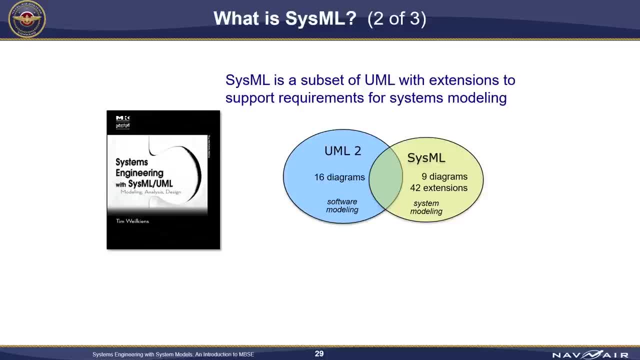 SysML is a subset of UML that has fewer diagram types but also has numerous extensions specific to systems engineering. This kinship between SysML and UML, that is, between systems engineering and software engineering, is particularly useful for systems that include software. 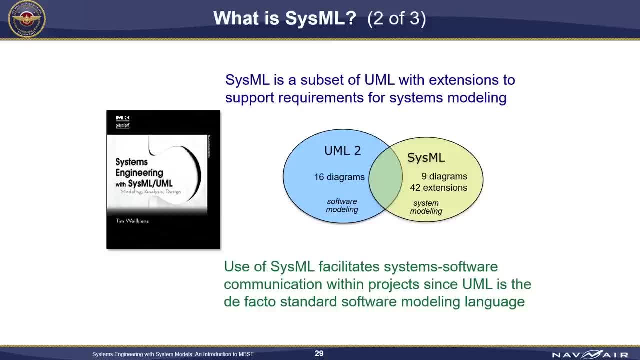 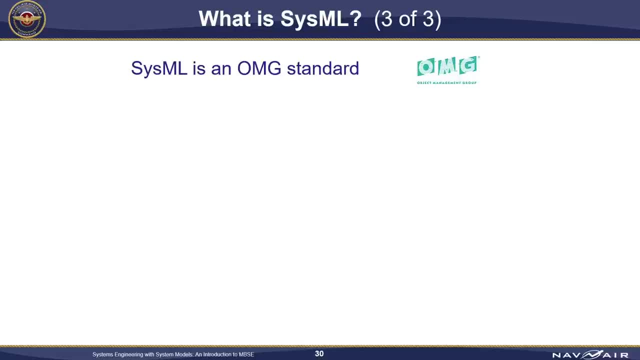 which is usually the case for the kinds of systems that NAVAIR develops and procures. Earlier we saw a quote from SysML that says that SysML is an industry-standard language. More specifically, SysML is a standard of OMG, the Object Management Group. 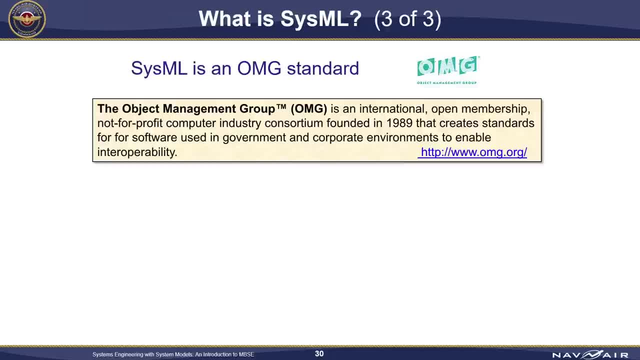 OMG is an international consortium that has developed specifications in various domains, including business process modeling, software modeling, system modeling, real-time middleware and many more. Note that their purpose in developing standards is interoperability, which is especially important for projects that involve multiple centers. 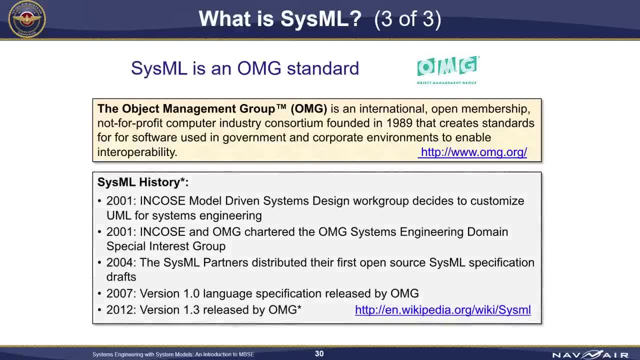 and multiple partners. Regarding SysML specifically, as this box shows, the history dates back to 2001,, when Nkosi decided to customize UML for systems engineering, thereby building upon a modeling language that began evolving in the 1990s. 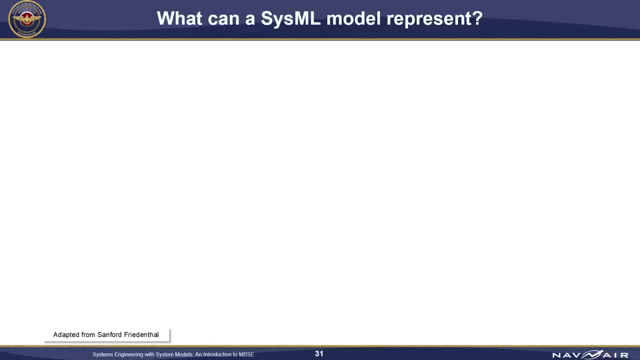 What can a SysML model represent? Well, first, it can represent various aspects of structure, including composition. For example, an EGI is part of an aircraft. It can represent interconnection, For example, the engines are connected to the engine control unit. 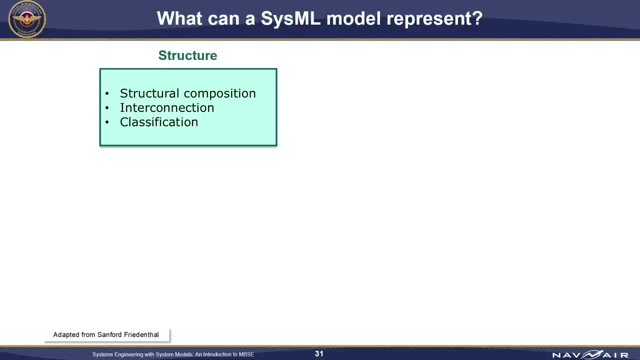 And classification. For example, an antenna is a type of flight hardware component. Next, a SysML model can represent behaviors in different ways. An example of function-based behavior is that an EGI provides attitude information. An example of message-based behavior is that a fault monitor emits a message. 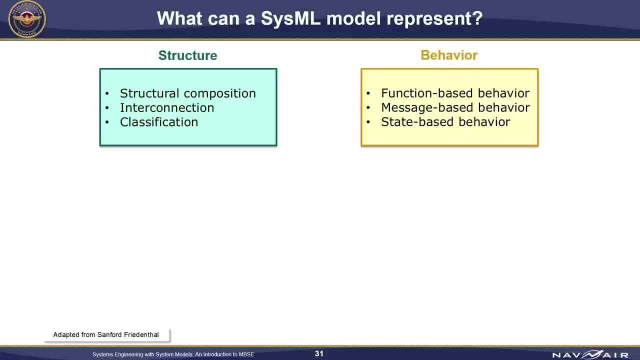 when it detects a problem, And an example of state-based behavior is that a radio transmitter transitions to an idle state upon receiving a certain command. Next, a SysML model can represent constraints on physical and performance properties. For example, it can represent the equation for calculating signal-to-noise ratio. 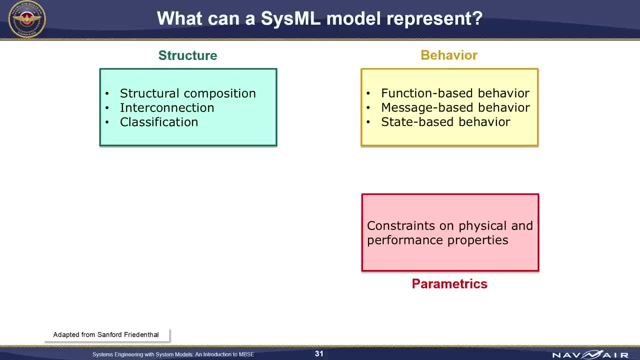 given values for all of the variables. Also, a SysML model can represent requirements and the relationships they have to other model elements, such as other requirements, components, interfaces, analyses and test cases. For example, consider a requirement that specifies that a component 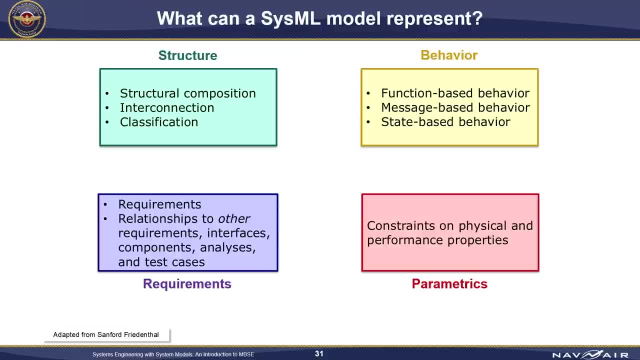 must provide a particular kind of interface. That requirement is a model element And it is explicitly related to the interface, which is another model element. In fact, there are many explicit relationships among model elements within a SysML model as depicted by these lines. 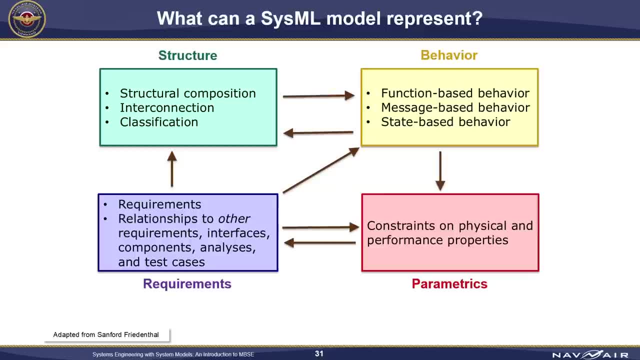 And that's essential to helping maintain consistency among the four categories of information shown here. Finally, just to keep things in perspective, none of these categories of information are new with SysML. To the contrary, they have always been part of systems engineering. 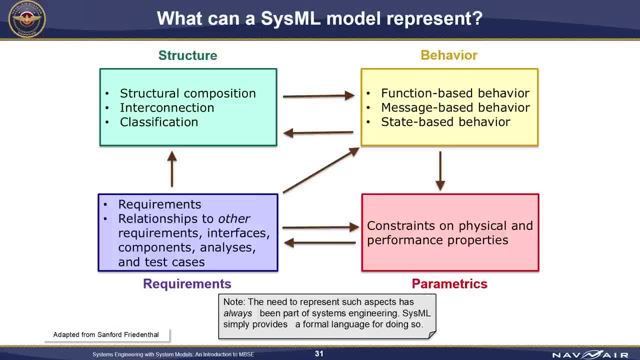 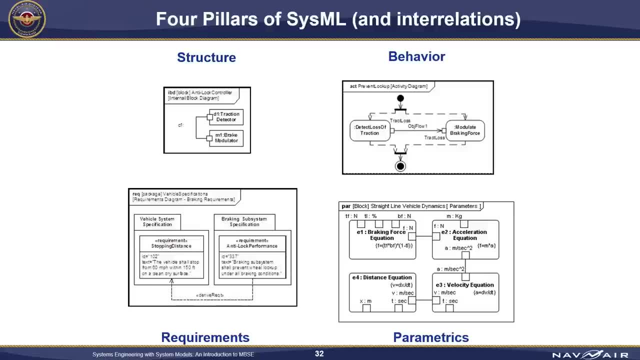 SysML simply provides a formal language for representing them, And SysML tools provide a way to help manage them. At the beginning of this module, we said that there would be a simple introduction to SysML, and most of it is on this one animated slide. 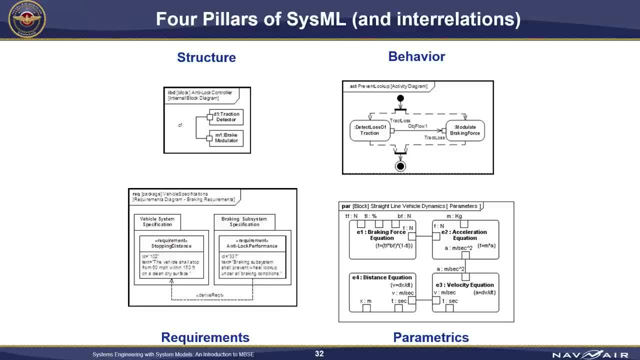 The first thing to note is that a system model consists of model elements that represent key aspects of design, including structure, behavior requirements and parametrics, each having their own diagrams. The example shown here is for an anti-lock brake controller for an automobile. 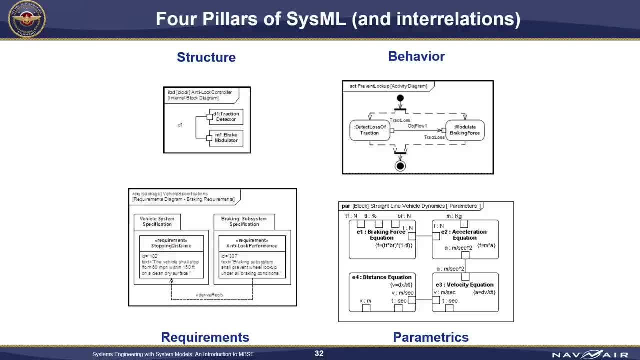 And under structure, we see an internal block diagram showing that the controller has a traction detector and a brake modulator and that they are connected together. Under behavior, we see an activity diagram showing two actions, namely detect loss of traction and modulate braking force. 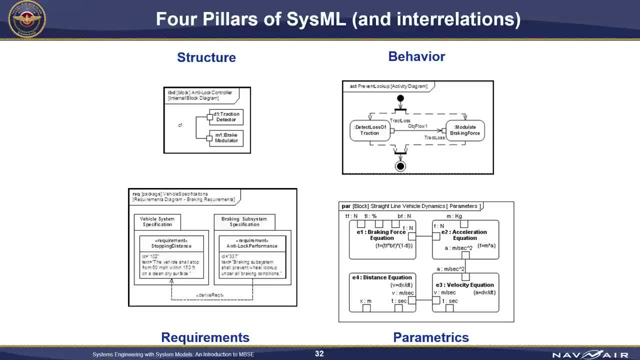 As we continue, we'll see the ways in which these diagrams are interrelated. For instance, we now see that each action has been allocated to a specific part of the controller, as shown in the red lines. Specifically, the action: detect loss of traction. 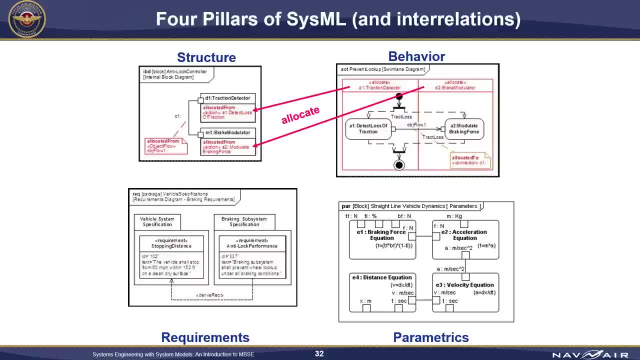 has been allocated to the traction detector and modulate braking force has been allocated to the brake modulator. Thus we're seeing the relations between a structural view and a behavior view of a system. Moving down to requirements. now we see that a requirement on anti-lock performance 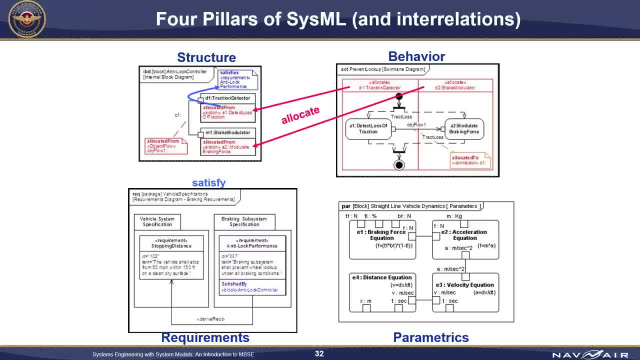 is satisfied by the anti-lock controller, or at least that's the claim. So let's see how that claim might be verified. Looking at the brake modulator, it has a value property called duty cycle. represented as a percentage, The value of duty cycle is bound. 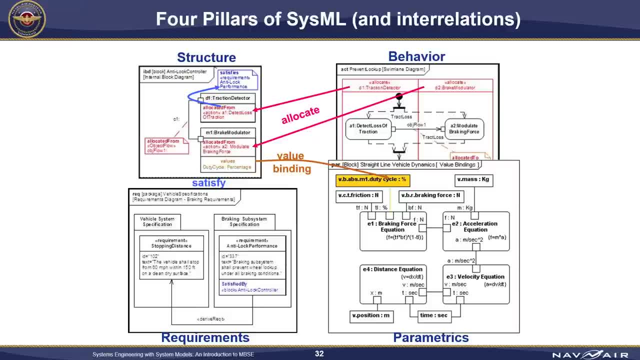 to the duty cycle parameter, which is an input to the braking force equation in parametrics. When all the inputs to all the equations have been supplied by other model elements which are not shown here, then the equations can be solved, yielding an output for vehicle position. 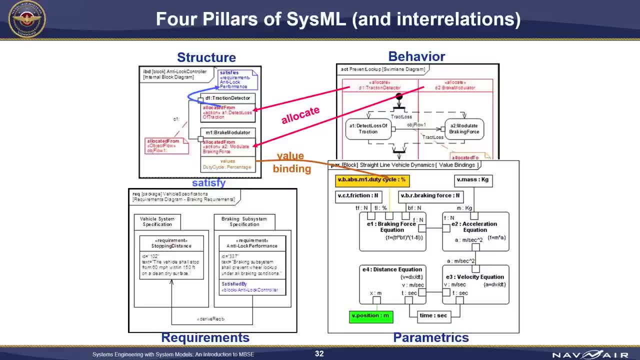 which is the same as stopping distance. That value can then be compared to the required minimum stopping distance to verify whether the design satisfies the requirement. Now, stepping back from the details, the kinds of connections shown in this slide exist in conventional systems engineering. 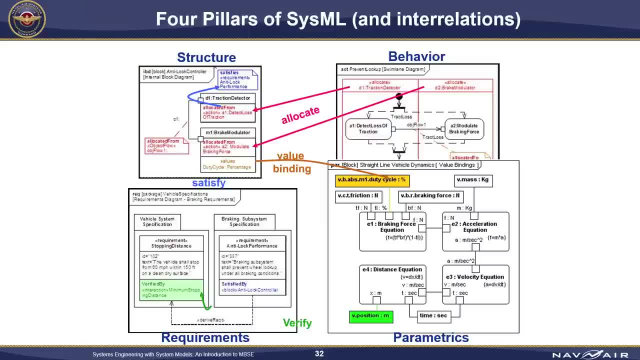 of course, but the actual connections themselves are more manual and typically involve different tools for text documents, diagrams and spreadsheets, And keeping all those artifacts mutually consistent requires discipline. What's different in using SysML is that the relations among model elements exist in a database as part of the system model. 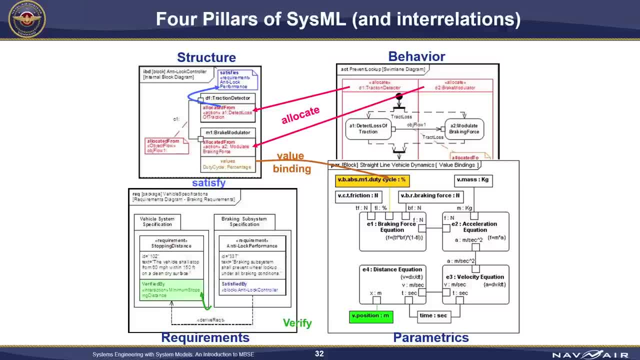 and that database can be checked for various types of consistency and completeness. Later we'll say more about the kinds of processing that can be done on a system model. In this section we've talked about what SysML is, but it's worth mentioning three things. 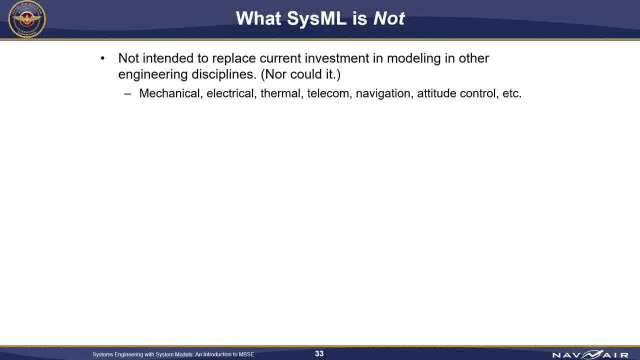 that SysML is not First. SysML is not intended to replace or subsume modeling and other engineering disciplines. Those disciplines, such as mechanical, electrical, thermal, etc. all have tools that are better suited for detailed modeling in their discipline. 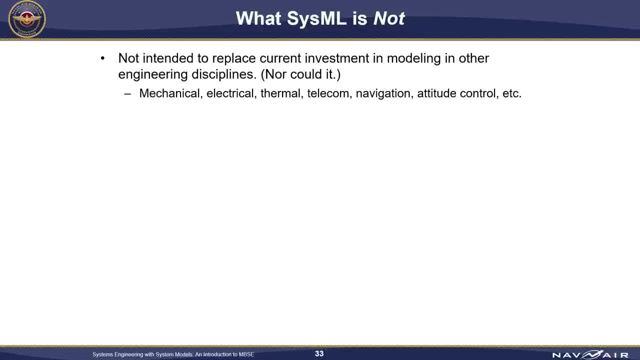 Modeling in SysML is intended to capture a more abstract system level of description. Second, SysML is not a methodology or a tool. It's a language and it is methodology-neutral and tool-independent. Third, although SysML is designed to support MBSE, 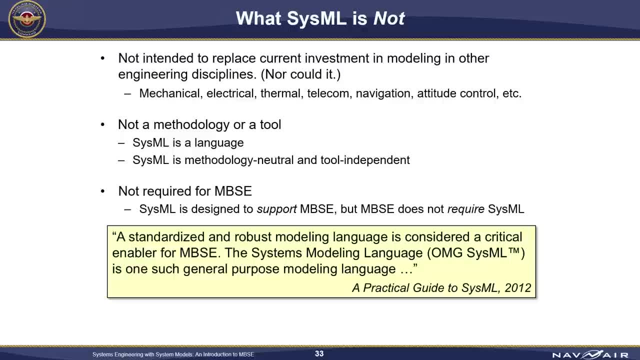 MBSE does not require SysML. This quote from one of the SysML books makes the point that a standardized modeling language is an enabler for MBSE and that SysML is one such modeling language. So this training module uses SysML. 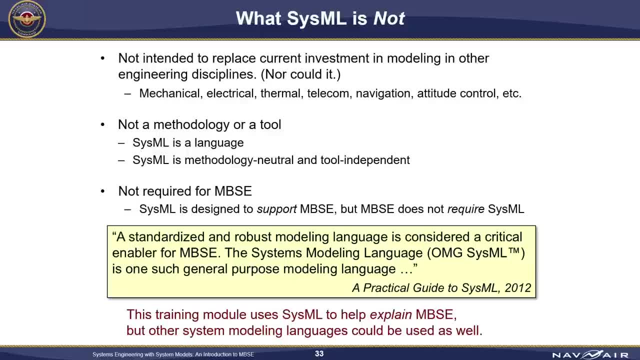 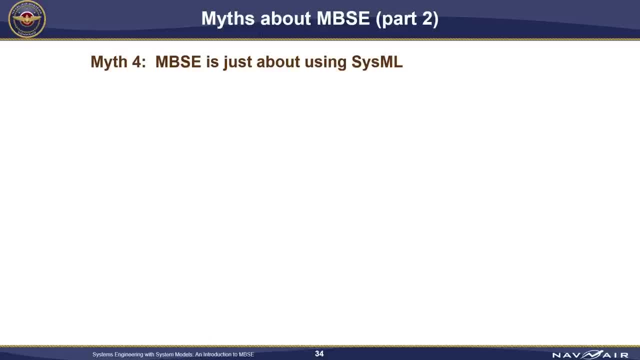 to help explain MBSE, but other modeling languages could be used as well. Let's now look at another myth: the myth that MBSE is just about using SysML. That's not true. SysML is a modeling language that can be used to describe systems. 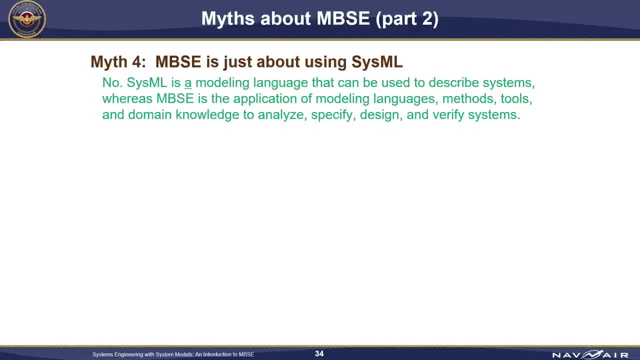 whereas MBSE is the application of modeling languages, methods, tools and domain knowledge to analyze and characterize the design. Another myth is that there's nothing really new in MBSE System. engineers already create many kinds of models. Well, of course it's true. 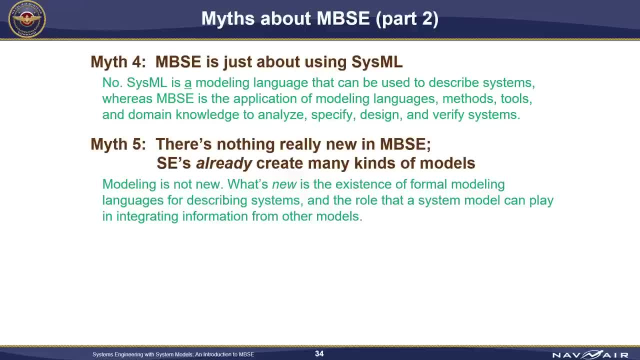 Modeling is not new. What's new is the existence of formal modeling languages for describing systems and the role a system model can play in integrating information from other models. Another myth is that SysML tools are just new drawing tools similar to the Visio and PowerPoint tools. 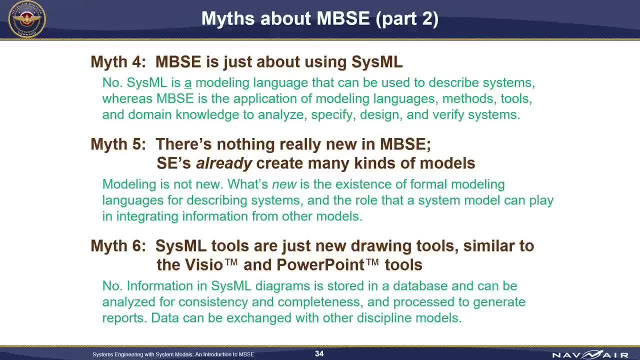 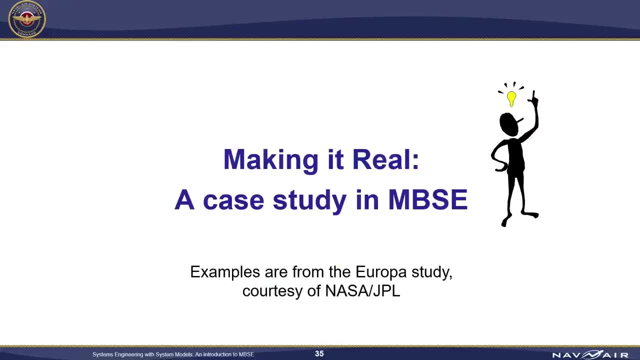 And that's not true, because the information in SysML diagrams is stored in a database and can be analyzed for consistency and completeness and processed to generate reports. Data can be exchanged with other discipline models from that database. Okay, let's move now to looking at case studies. 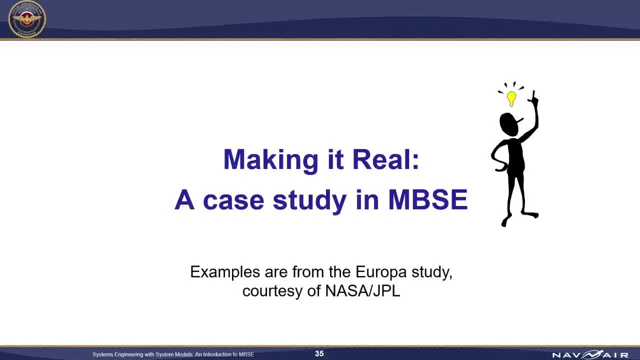 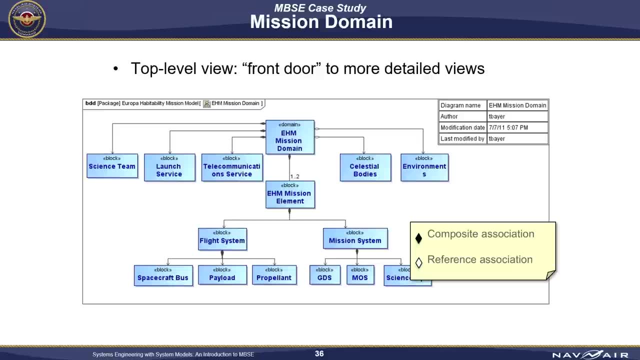 These case studies come from the Europa study, courtesy of NASA, JPL. This simple block diagram in SysML is a structure diagram that shows the mission domain for the EHM. EHM stands for Europa Habitability Mission, and that mission domain is composed of several elements. 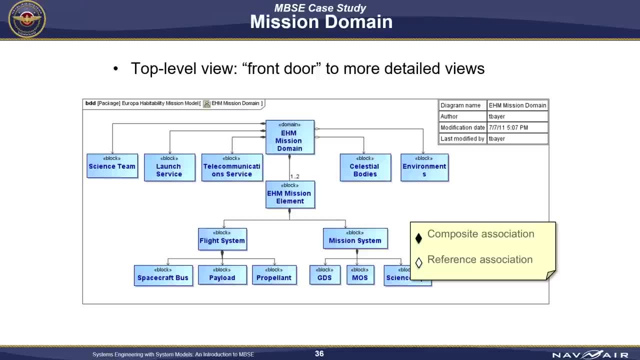 including the science team, launch service, telecommunication service and mission elements. The mission element further decomposes into the flight system and the mission system And, as you can see, the flight system is further decomposed, as is the mission system. 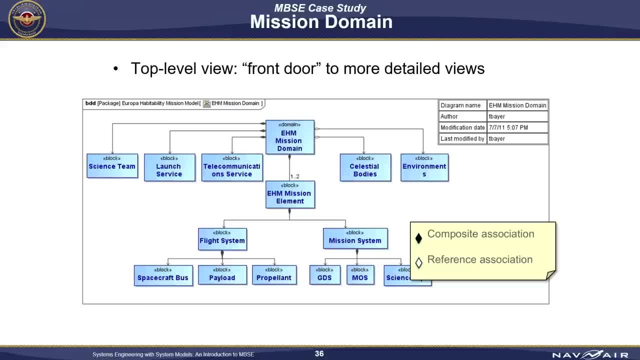 What's useful about this kind of diagram is that it can serve as a top-level view or front door to the system model. Clicking on blocks in this diagram leads to more detailed views. This diagram sometimes referred to as a system block diagram. 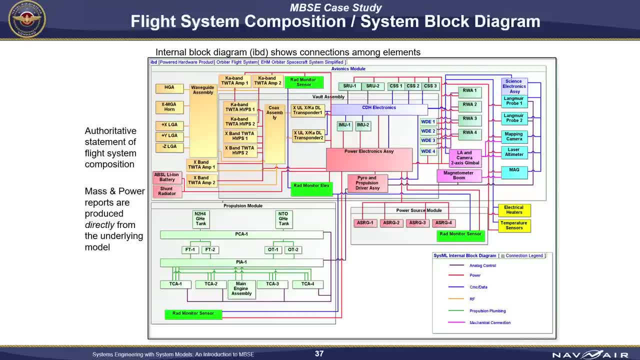 is also a SysML diagram. Visually it looks very much like the kind of diagram that engineers have produced in PowerPoint or Visio, But in SysML all these modeling elements and the connections among them are represented in a database. 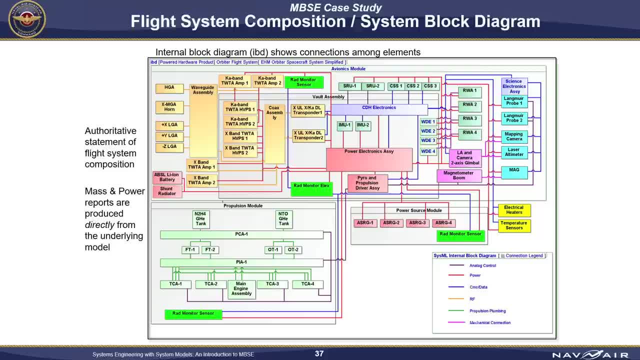 As you can see in the connection legend in the lower right, different types of connections are shown in different colors and that's for the benefit of people reading the diagram In the database. those connections are distinguished with different classifiers, A key point discussed previously. 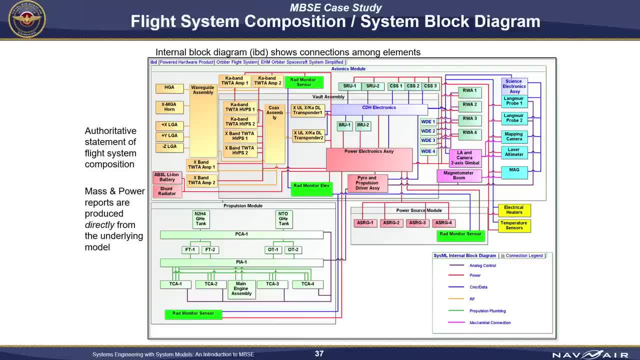 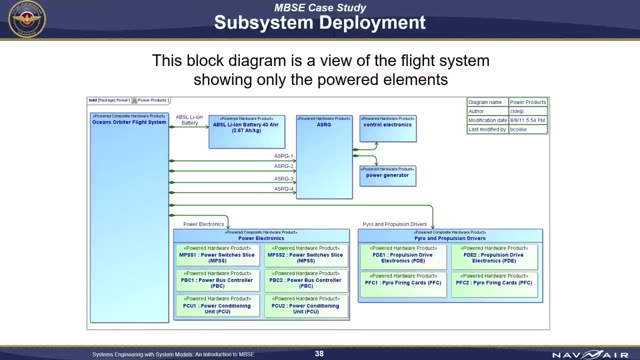 is that such a model can be analyzed in various ways, using algorithms that traverse the database, extracting what's needed for the analysis. This block diagram is a kind of structure diagram in SysML that shows what is connected to what, In contrast to the previous diagram. 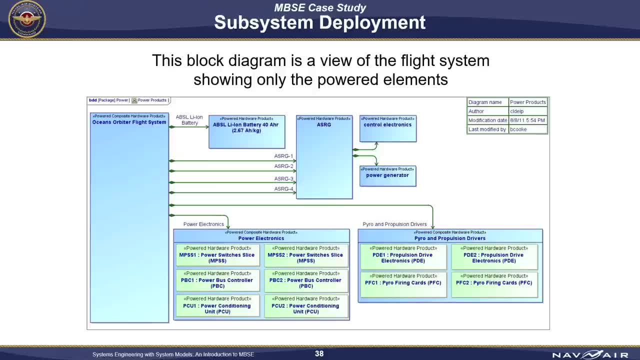 that showed components and connections. this block diagram shows a couple of levels of decomposition but no connections. For example, the Oceans Orbiter Flight System block shown on the left is composed of a battery, an ASRG power electronics and pyro and propulsion drivers. 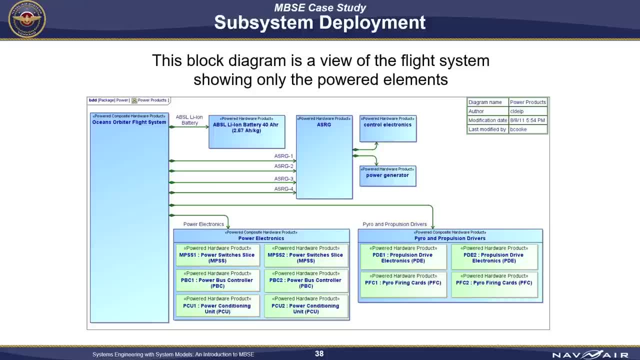 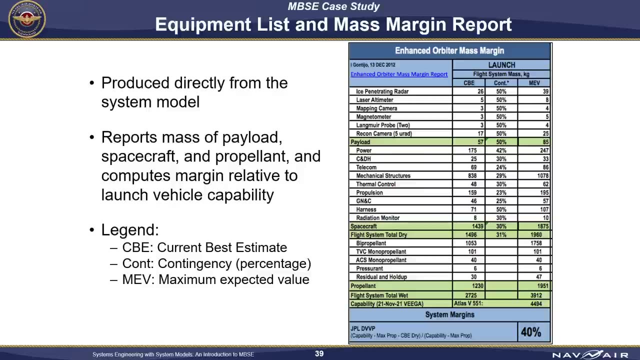 Those last two are further decomposed into other products. So this block diagram is a kind of structure diagram in SysML that shows what is part of what. This slide shows a simple example of a report that can be generated from information in the system model. 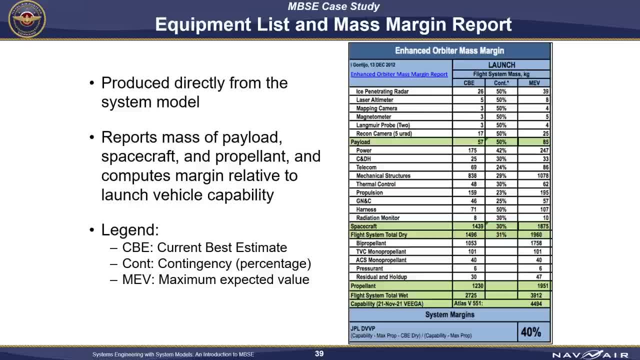 It shows the current best estimate of mass for different parts of the spacecraft and the maximum expected value. The report rolls up the total mass of the payload, the spacecraft and the propellant and computes the margin relative to the launch vehicle capability. It's a simple example of a common view. 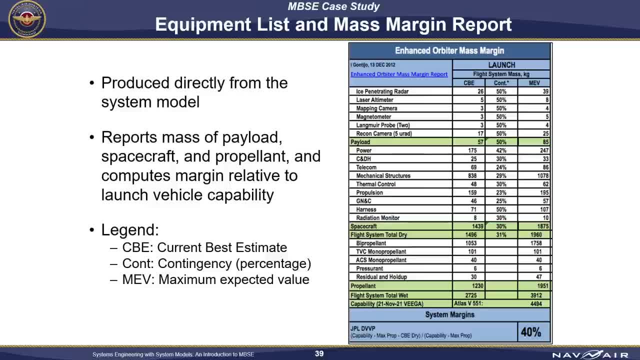 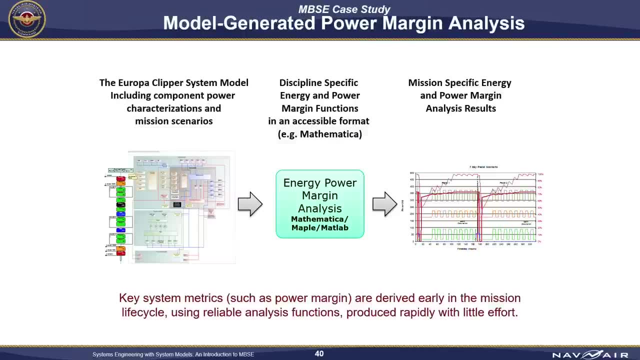 of the design. that's really important to some stakeholders. What's important to keep in mind is that, as long as the system model is kept up to date with mass information, this kind of report can be regenerated easily and frequently. This slide shows an overview of how. 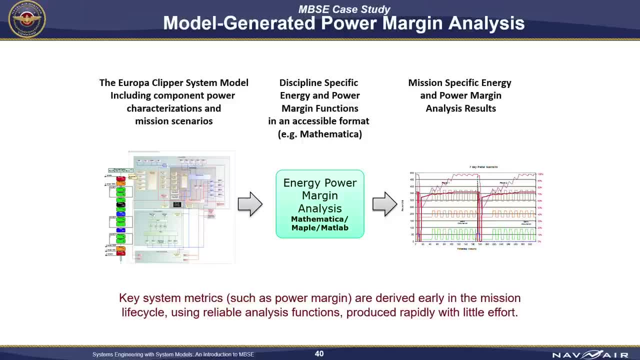 a power margin analysis is generated In simple terms. information in the system model about component power loads and mission scenarios is provided to an analysis program that computes how power and energy changes over the course of one orbit around Jupiter, which takes seven Earth days. 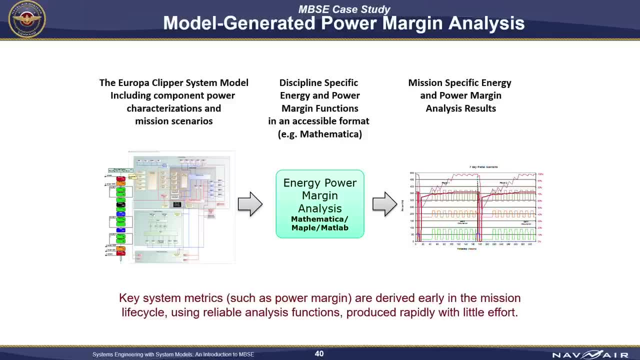 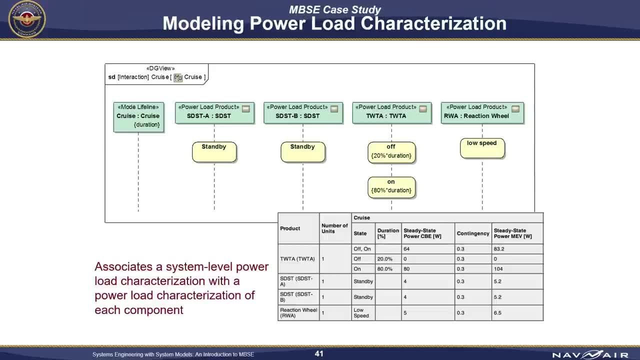 The analysis program in this case was developed in Mathematica, but other mathematical tools could be used. This chart shows the power modes of different spacecraft elements, such as transponder, traveling wave tube and reaction wheel. The power modes are shown in a sequence diagram. 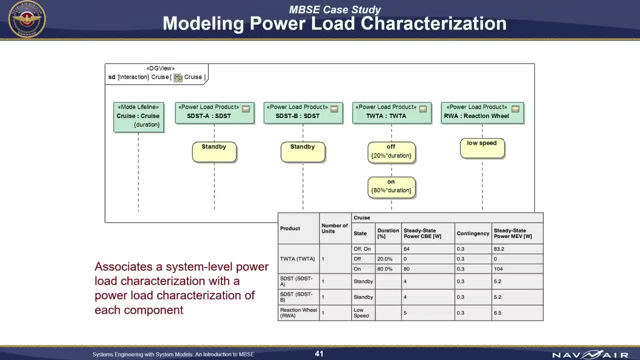 and each such mode has an associated power draw in watts, as shown in the table on the bottom right. This information will be used in the next step when we look at all the different segments of a seven-day orbit, The next part of power margin analysis. 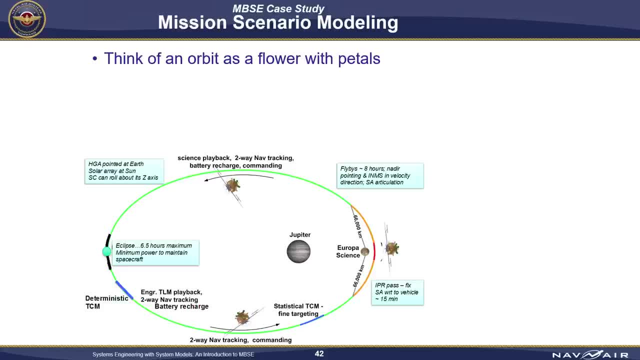 requires representing a mission scenario: an orbit around Jupiter that flies past Europa as a sequence of system modes, each having its own details about energy production and power consumption. Each orbit around Jupiter takes seven Earth days, and that orbit can be thought of as the petals of a flower. 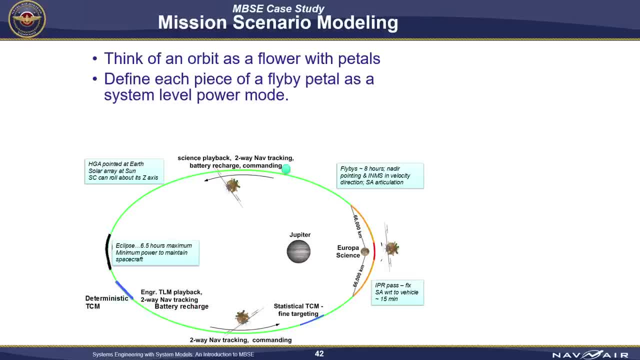 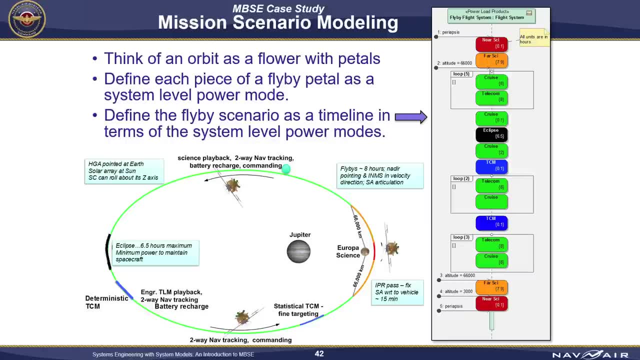 Each petal represents a system-level power mode and, as we see here on the right, the scenario starts at the top with a red petal for what's called near science, and then an orange petal for far science, and then green petals for cruise and telecom. 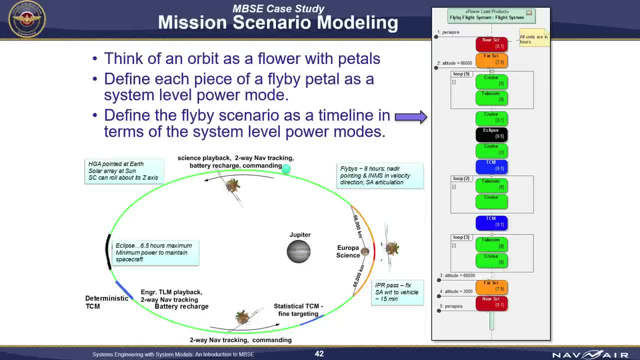 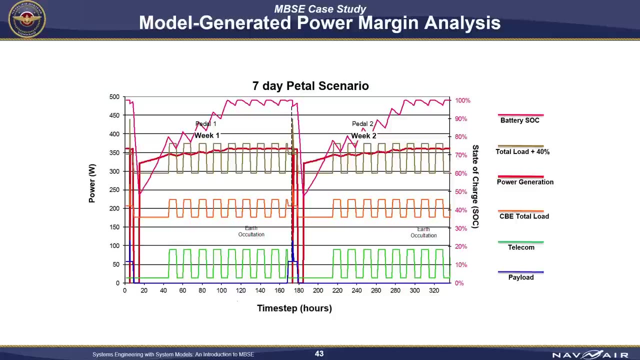 and so forth. With that, including the time duration for each petal, we now have enough information in the model to calculate the power margin analysis. This slide shows the results of the analysis for two consecutive orbits. Using the legend on the right, 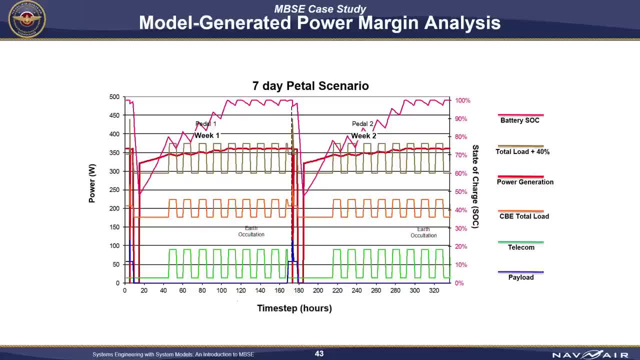 we see the green line showing periods of telecom activity. We also see the red line showing power generation, which is fairly constant except during eclipse, And the pink line shows battery state of charge, which declines sharply during eclipse and gradually builds back up to 100%. 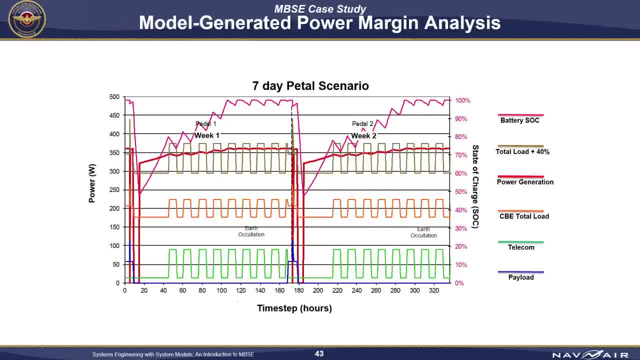 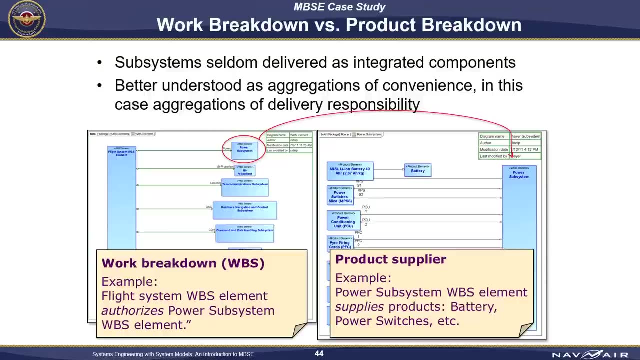 before the next eclipse. Although the power model used here is quite simple, it enables the project to do a margin analysis and easily recalculate it as the design changes. This chart shows the distinction between the work breakdown, shown on the left, and a product supplier, shown on the right. 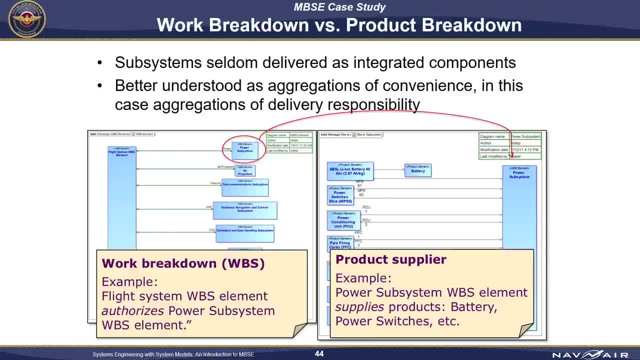 Subsystems are seldom delivered as integrated components. They are better understood as aggregations of convenience, In this case aggregations of delivery responsibility. So what we see on the left is the work breakdown element of power subsystem and over on the right 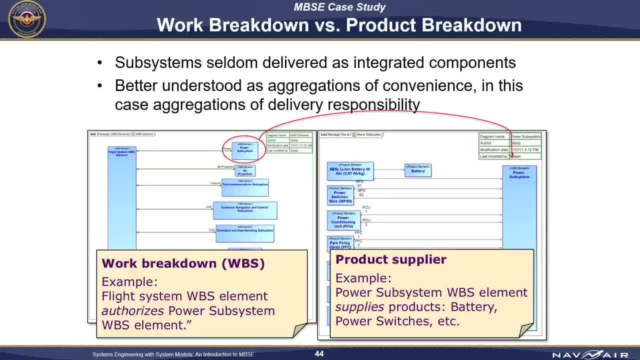 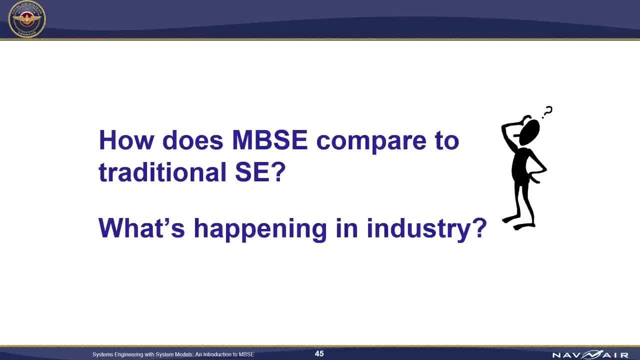 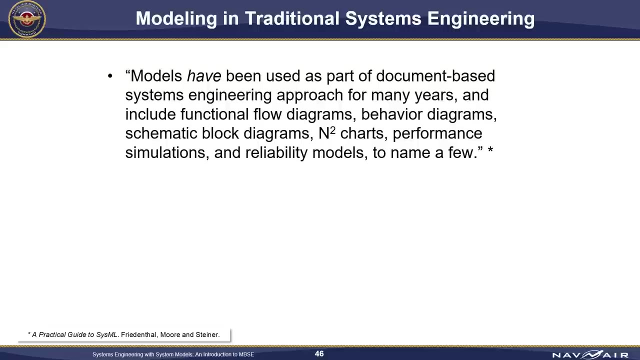 we see that the power subsystem work breakdown element is responsible for different products in the product breakdown. Now let's ask the obvious questions: How does MBSE compare to traditional SE And what's happening in industry? Models have been used as a part of a document-based systems engineering approach. 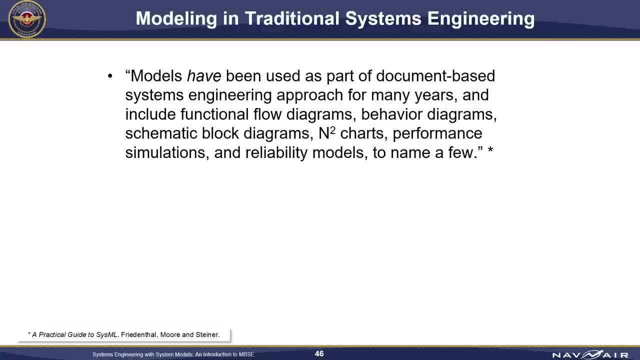 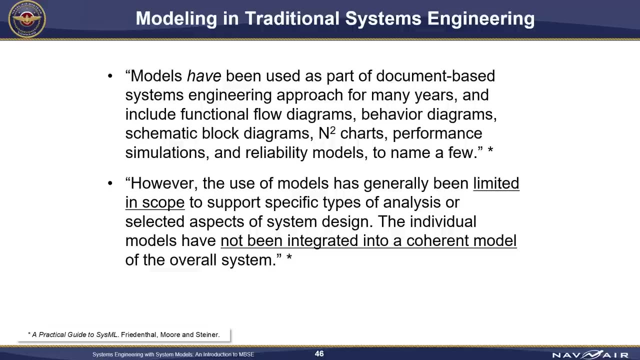 for many years and include functional flow diagrams, behavior diagrams, schematic block diagrams, n-squared charts and others. However, the use of models has generally been limited in scope to support specific types of analysis or selected aspects of system design. The individual models have not been integrated. 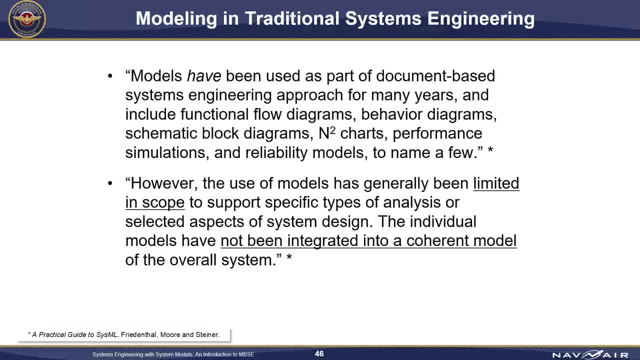 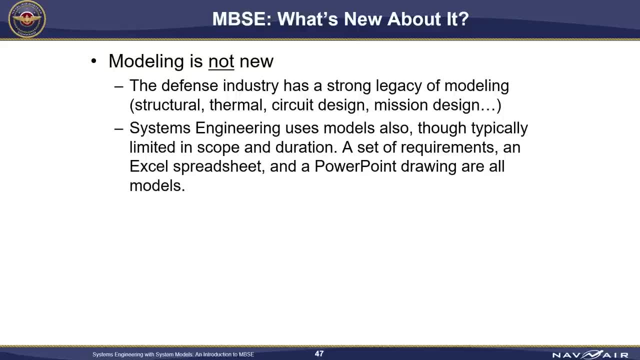 into a coherent model of the overall system. So what's new about MBSE? Certainly, modeling is not new. The defense industry has a strong legacy of modeling Systems. engineering uses models also, though typically limited in scope and duration. A set of requirements: 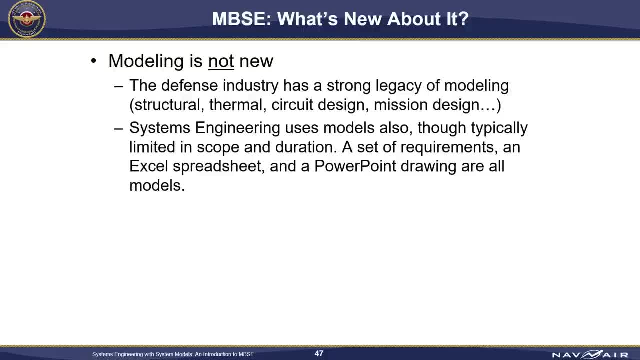 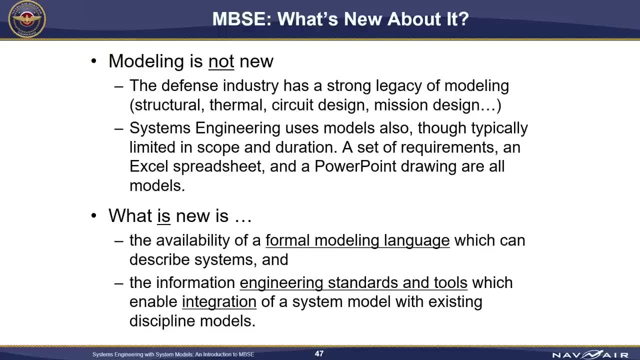 an Excel spreadsheet and a PowerPoint drawing are all models. in a sense, What is new is the availability of formal modeling languages which can describe systems and the information engineering standards and tools which enable integration of a system model with existing discipline models. 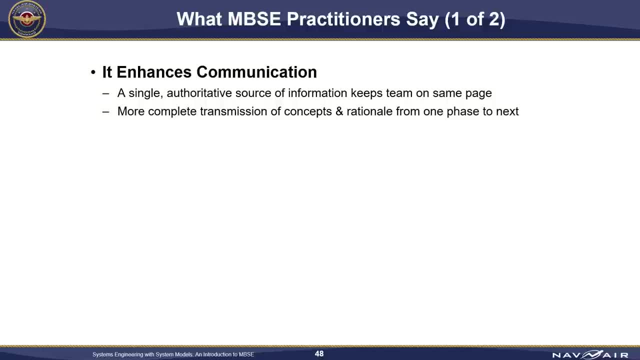 Now let's look at some examples of what MBSE practitioners are saying. This is what we've heard from various practitioners applying MBSE on different types of projects. Most commonly, we hear that it enhances communication. There is a lot of benefit to having a single authoritative source of information. 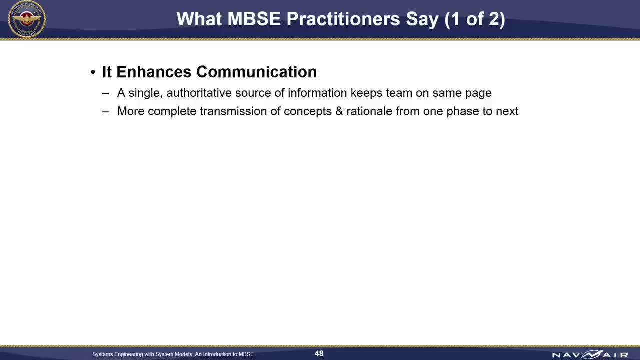 that keeps the team on the same page And there is a more complete transmission of concepts and rationale from one phase of the project to next. It also improves productivity. There is less hunting for information and time-consuming project documents and reports become trivial to generate. 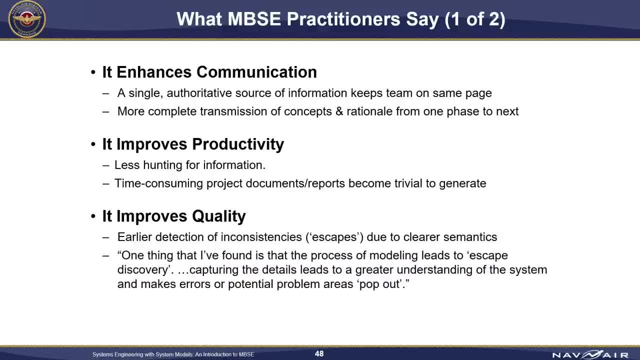 It improves quality. We often hear there is earlier detection of inconsistencies or escapes due to clearer semantics and just the act of modeling. One practitioner said One thing that I've found is that the process of modeling leads to escape. discovery, capturing the details leads to a greater understanding of the system. 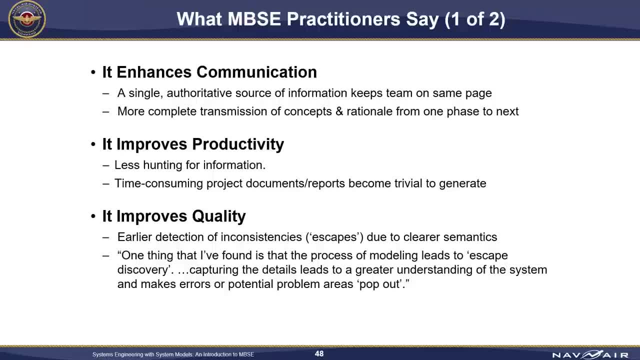 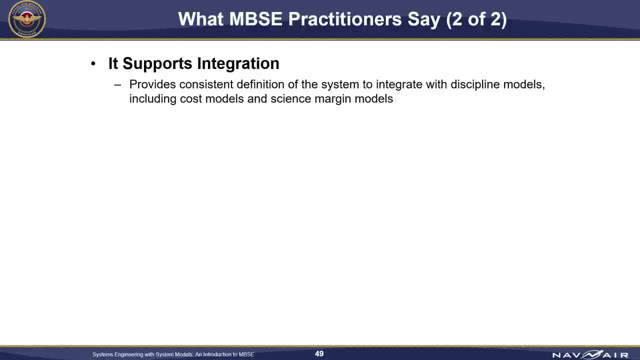 and makes errors or potential problems pop out. Other practitioners say MBSE supports integration. It provides consistent definition of the system to integrate with discipline models, including cost models and science margin models. It helps manage complexity. Different views address the concerns of different stakeholders. 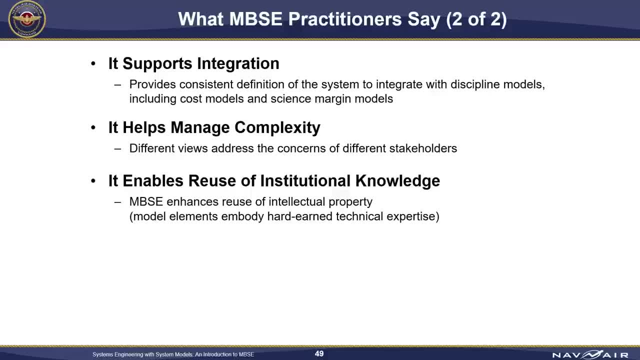 It enables reuse of institutional knowledge. MBSE enhances reuse of intellectual property because the model elements embody a lot of hard-earned technical expertise and the analyses that go with it. It attracts early career talent. MBSE forms a bridge from their college education to institutional practices. 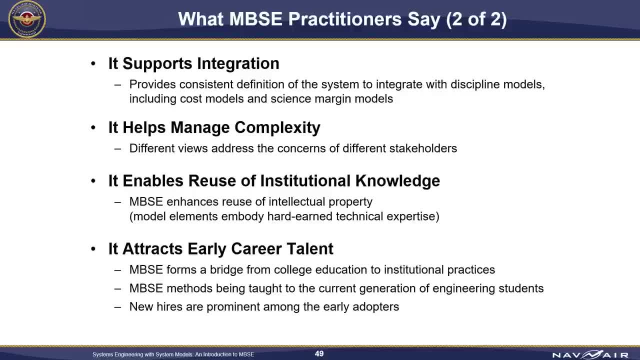 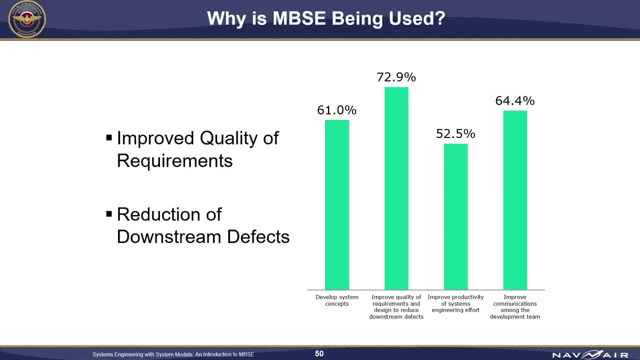 MBSE methods are being taught to the current generation of engineering students, and we see that new hires are prominent among the early adopters. As to why MBSE is being used, a majority cited the opportunity to improve systems engineering efforts as the reason for using modeling. 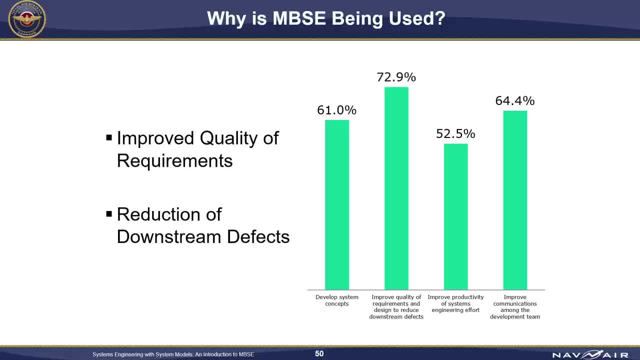 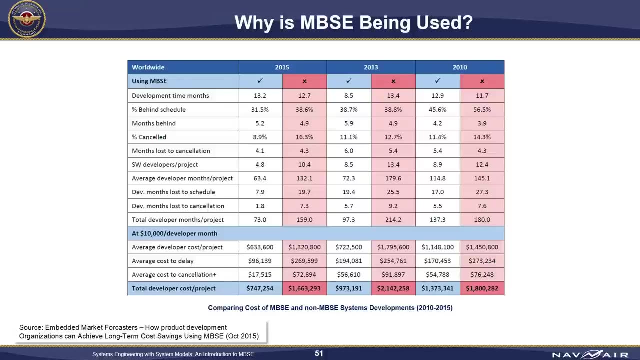 And when they were asked about the primary purpose of the model, the majority said that it was specifically to improve the quality of requirements and design to reduce downstream defects. From this improvement in the quality of requirements and reduction of downstream defects- it logically follows that both cost. 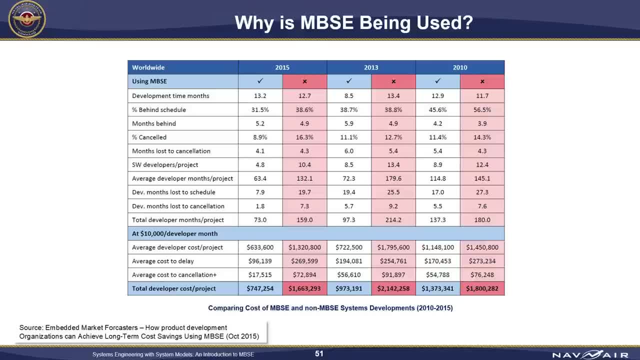 and schedule of programs using MBSE will be reduced. A sample of this reduction is shown in this chart, taken from a report published by Embedded Market Forecasters, a market research and consulting firm for embedded products. The data presented is taken from six years of EMF survey data. 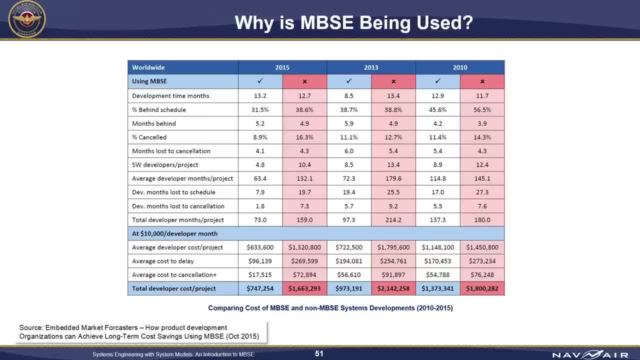 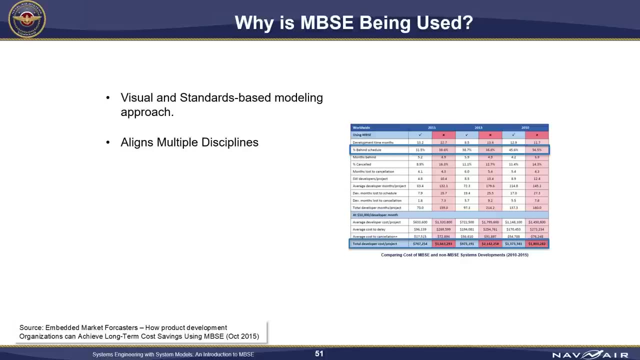 totaling more than 4,000 developer responses. As you can see, there were savings in both schedule and cost across all of the years surveyed. The report credits the advantage of a visual and standards-based modeling approach that aligns electrical, mechanical software and architecture. 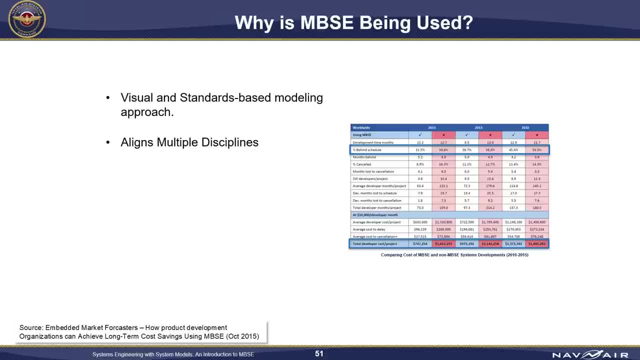 all of which use differing technology, language and tool sets, with a common whole-systems view of the product under development. It replaces ambiguity with clarity that transcends both engineering discipline and geographic location. Okay, let's recap. First, we've seen that MBSE formalizes part of SE. 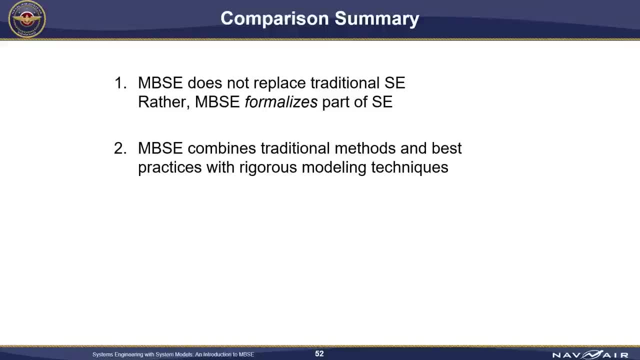 It doesn't replace it. Second, MBSE is still SE, so traditional methods of analysis and verification still apply, and some of them are facilitated by having a rigorous system model. Third, we get these benefits because formal system models help expose inconsistencies. 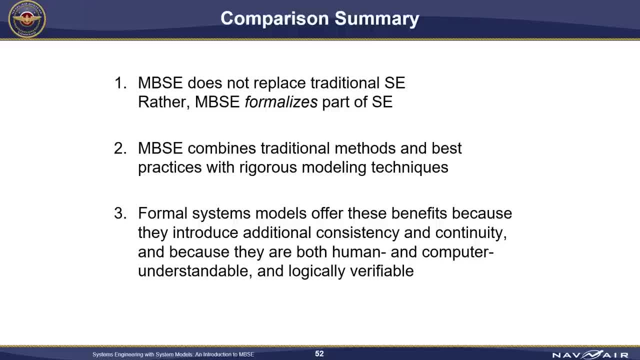 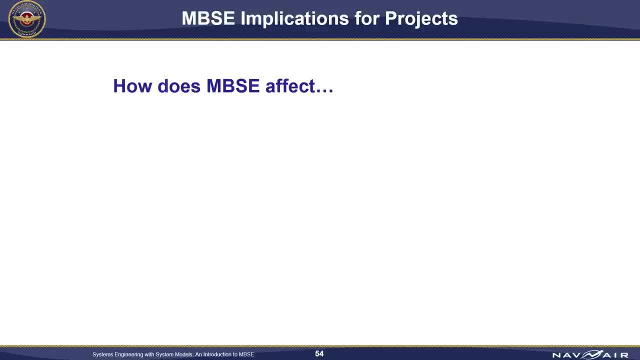 partly because they are human-understanding and partly because they are logically verifiable. Let's shift our attention now to some management issues. Let's look at how MBSE affects documents, project organization, processes, infrastructure and metrics- The context to answer these questions. 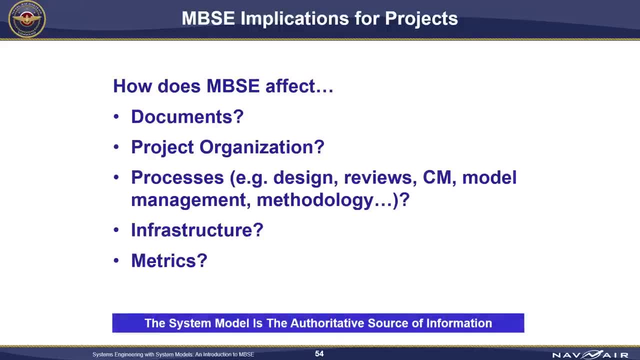 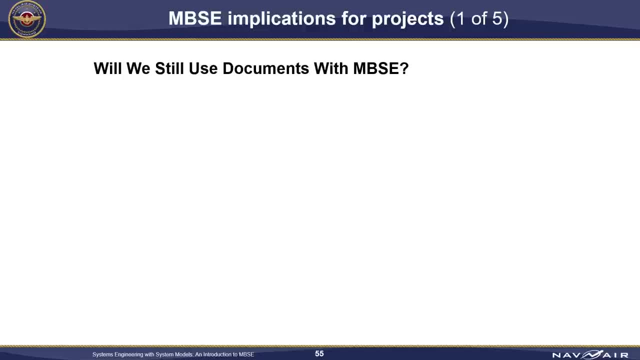 is that the system model is the authoritative source of information. Let's take these one by one. Will we still use documents with MBSE? While the intent is to shift from documents to model views, the project may still have to produce some documents and artifacts for reviews. 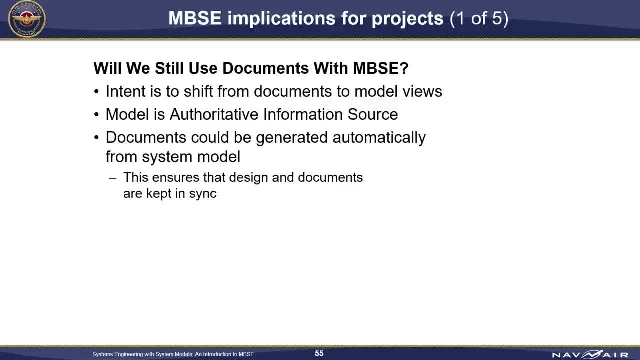 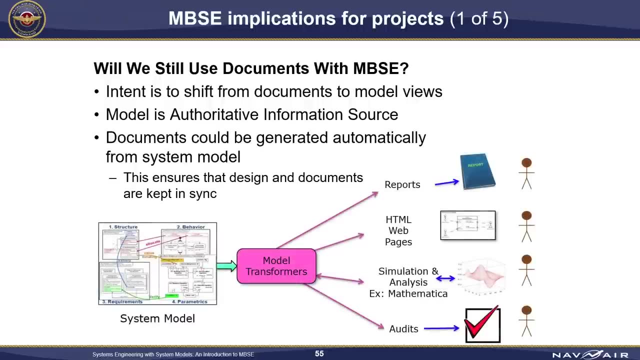 If a document is required, it should be able to be generated from the model, as the model is the authoritative source of information. This ensures that any documents prepared are consistent and in sync with the truth data. This diagram shows how model transformers can produce reports and webpages. 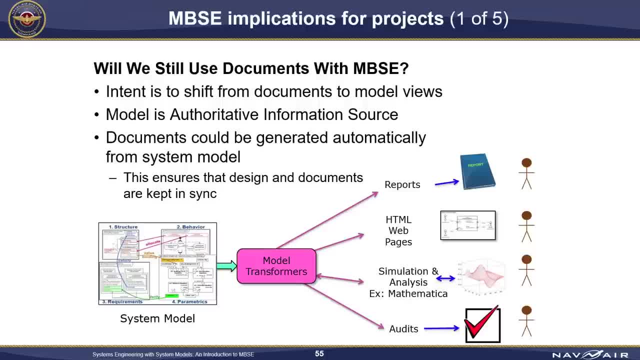 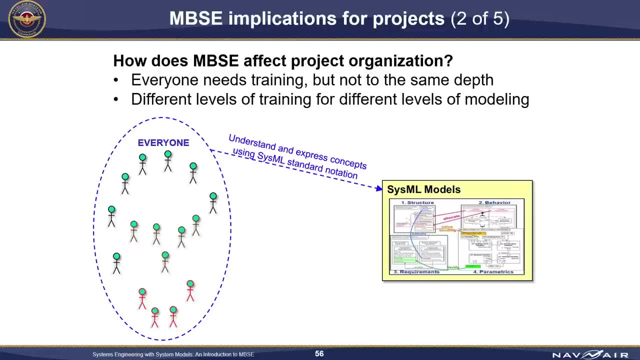 and can extract portions of the model for automated analyses and perform audits for consistency and correctness on the model, Audits that would otherwise require a lot of manual labor by humans. How does MBSE affect project organization? Well, in terms of training. Everyone needs training to some extent. 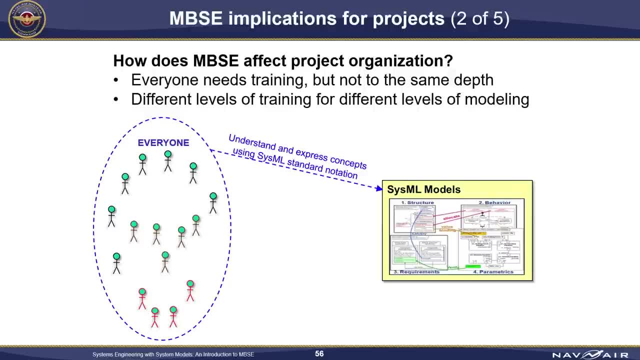 to understand the models, but not to the same depth. For example, we want everyone to understand and express concepts using SysML standard notation. Also, a smaller group of subject matter experts- most of them including the leadership- will collaborate, develop and review models. 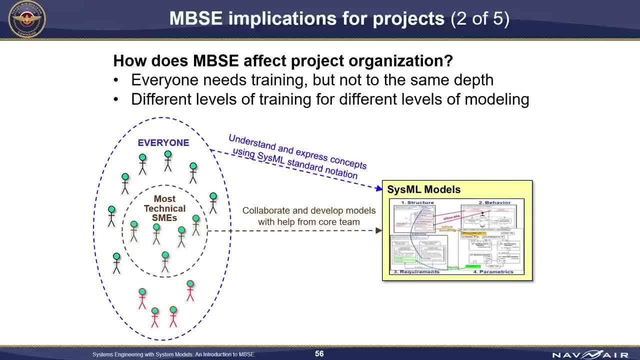 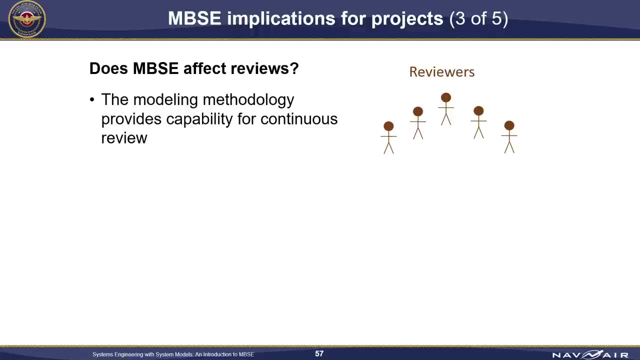 with help from the core modeling team. So they'll need a little more training in the use of SysML. And finally, the core modeling team will apply best practices and contribute to the production of models. Now, how does MBSE affect reviews? 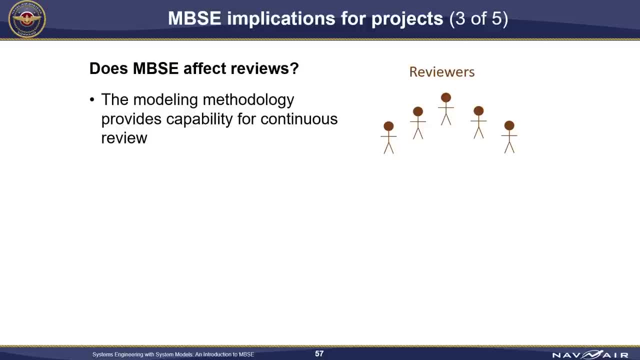 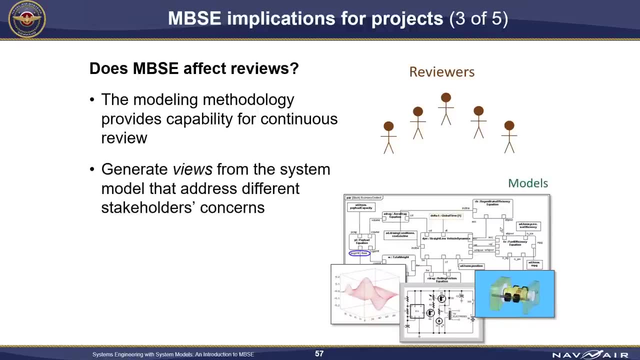 The modeling methodology provides the capability for continuous review and collaboration between government and contractor. What we can do is generate views from the system model that address different stakeholders' concerns, and we can leverage the model by reviewing the model itself, In other words, using the live model in a review. 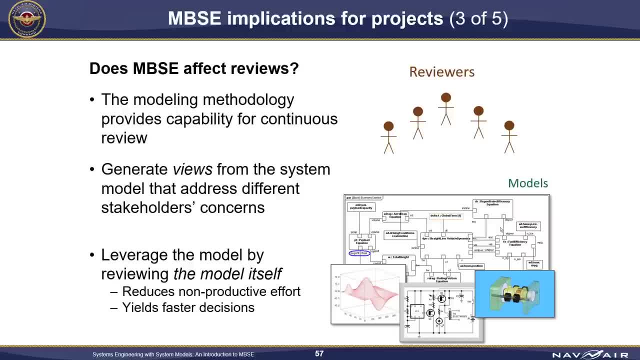 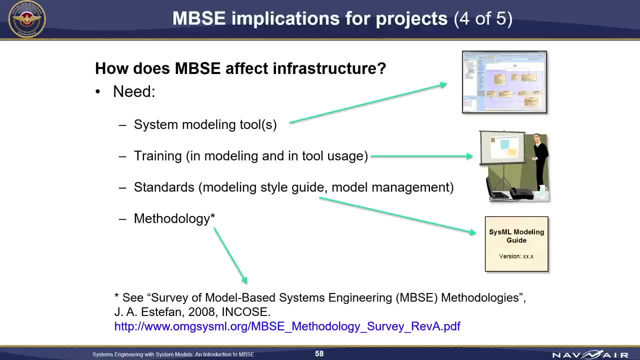 as opposed to static capture in PowerPoint diagrams. This reduces non-productive effort and yields faster decisions. Again, the model serves as the authoritative source. How does MBSE affect infrastructure? Pretty much in the ways you would expect You are going to need. 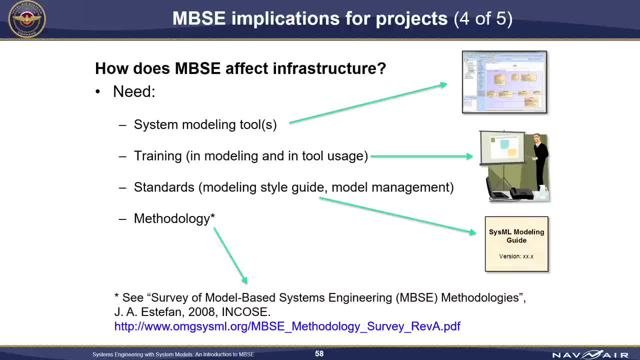 a system modeling tool, You'll need training, you'll need standards and you'll need methodology. This is pretty typical of introducing a new way of doing things or any modification thereof. How does MBSE affect metrics? It is easier to get data from models. 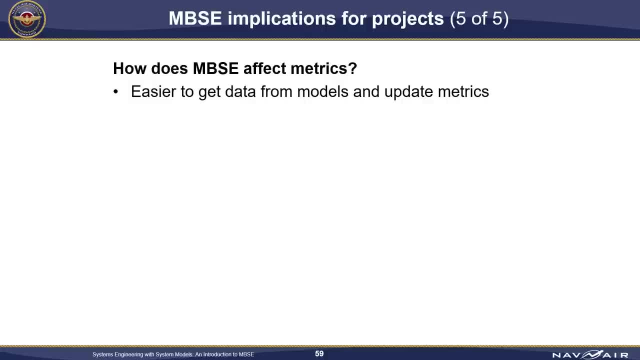 and update metrics, because if the information is in a well-structured system model, there are many kinds of metrics that can be collected and presented, For example, the quality of design in terms of weight margin, power margin, data margin, etc. The progress of the design. 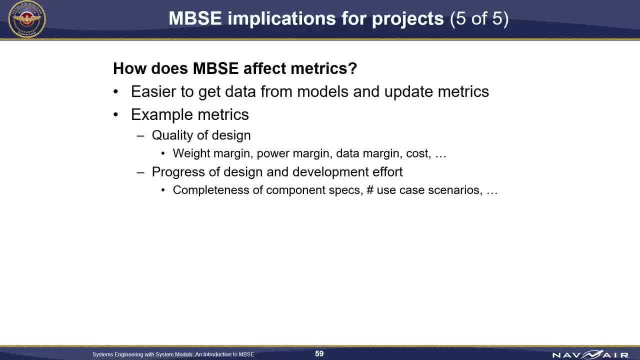 and development effort according to the completeness of component specifications, Estimated effort to complete the design and development, and various other types of metrics such as the number of critical TBDs and the stability of requirements and design changes over time. So all of these are possible. 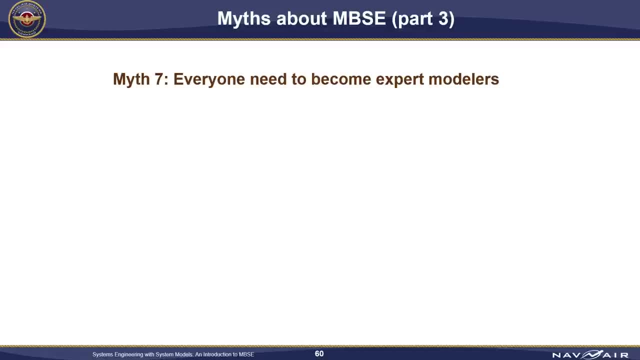 Now let's examine a few more myths about MBSE. One myth is that everyone will need to become expert modelers. The answer is no. You can establish a core modeling team to build the model, but we want all technical subject matter experts to be able to interpret the model. 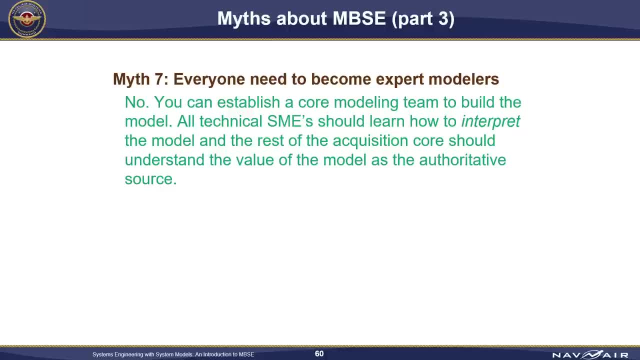 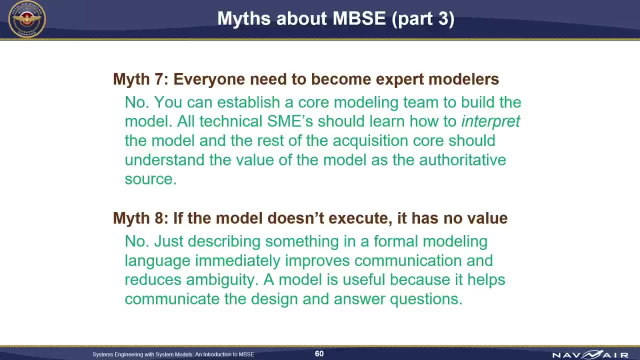 Also the remaining acquisition core needs to understand the value of the model as the authoritative source. Another myth is if the model doesn't execute, it has no value, And that's not true. Just describing something in a formal modeling language immediately improves communication. 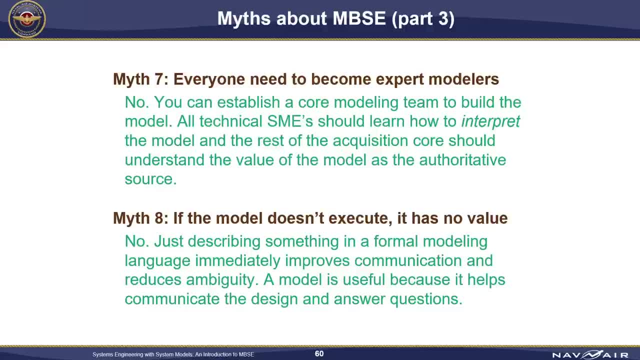 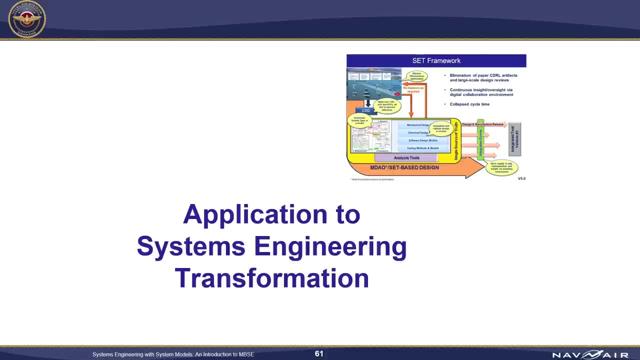 and reduces ambiguity. A model is useful because it helps communicate the design to answer questions, And this has been one of the findings in NASA's use of MBSE. So how does all of this apply to the NAVAIR Systems Engineering Transformation Initiative? 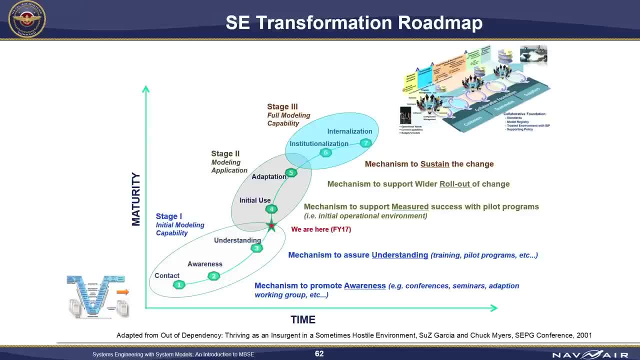 Culture change is certainly an issue to consider in moving from traditional engineering to a more model-centric approach. This slide simply shows the kind of changes that take place over time in changing the culture of an organization, From initial contact all the way through understanding. 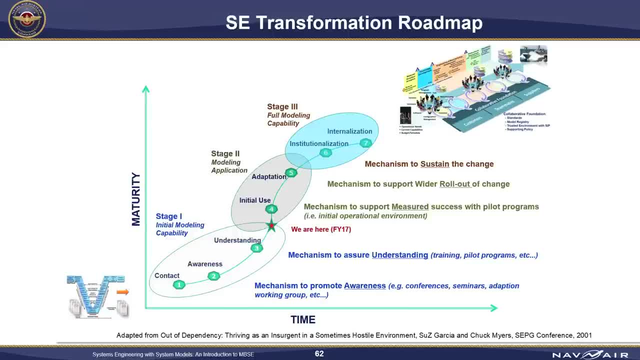 initial use and adoption and finally, institutionalization and internalization. This kind of culture change roadmap took place with mechanical and electrical computer-aided design years ago, And so systems engineering is going through this kind of roadmap. now Let's look at a multi-year strategy. 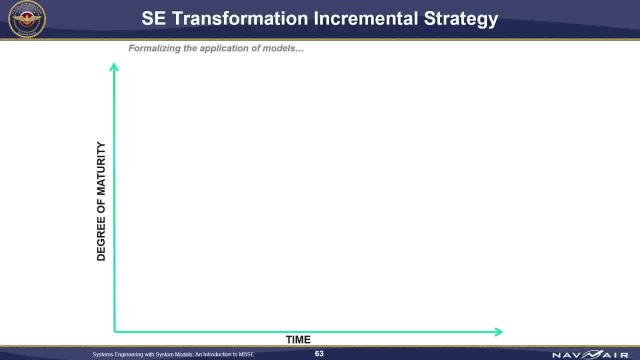 for deploying MBSE. Let's think of it in terms of three phases. The first phase is building. That is where we start training a set of MBSE modelers. provide modeling infrastructure that facilitates collaborative modeling activities. provide an initial modeling standard. 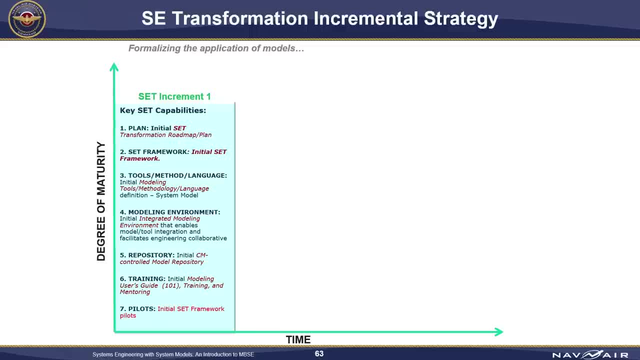 modeling user's guide and a CM-controlled model repository framework, and embark on pilot programs. A second phase, a little later in time, is where the key capabilities include tools, methods and language that are fully established and supported to facilitate technical assessment using models. 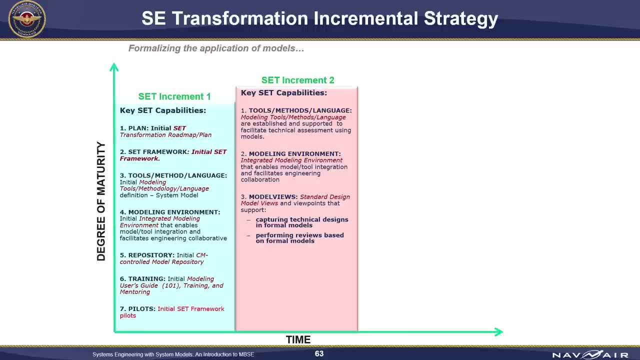 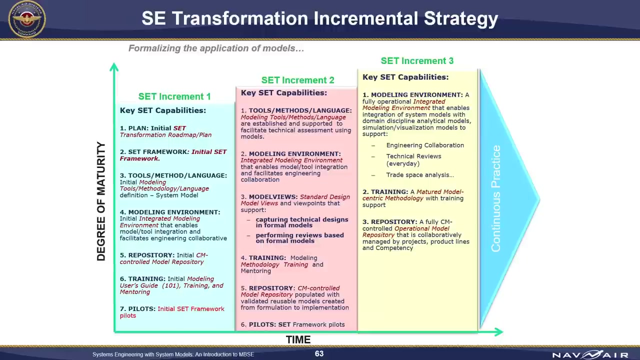 a modeling environment that enables model and tool integration and facilitates engineering collaboration, standardized model views, a well-established training method and curriculum. and a CM-controlled model repository with validated reusable models. Finally, in a third phase, a so-called integrating phase, the key capabilities would include: 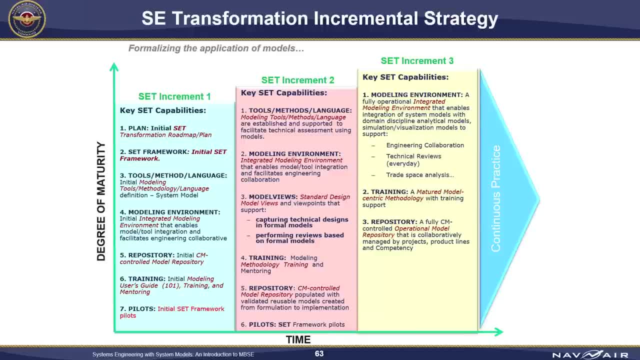 a fully operational modeling environment or infrastructure that enables the integration of system models with domain discipline analytical models, provides a mature model-based development methodology with training support. and, finally, provides a fully CM-controlled operational model repository that is collaboratively managed by projects lines and enterprise. 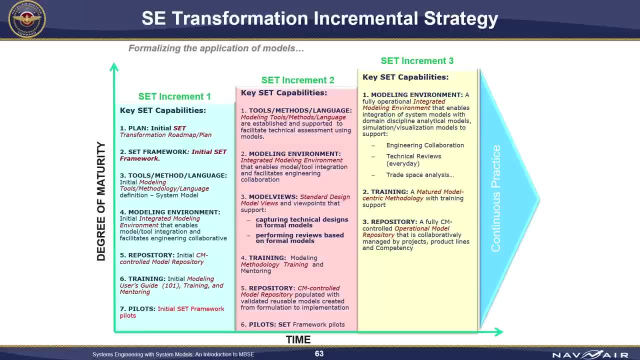 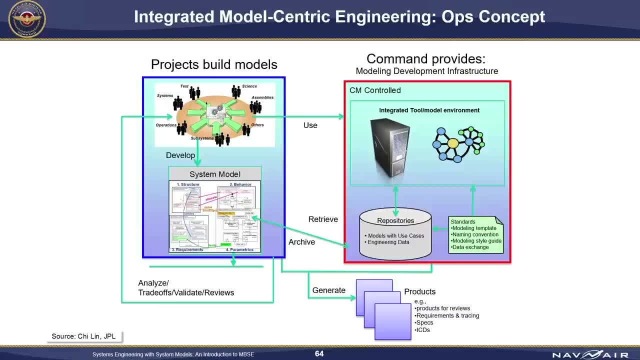 and that becomes continuing practice into the future In terms of integrated model-centric engineering. this slide depicts the operations concept we plan to use at NAVAIR. On the left we see the projects, of course, using a modeling tool to develop a system model. 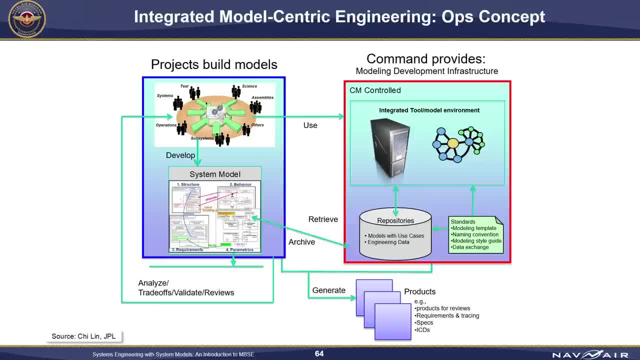 They will perform analyses, identify trade space, validate and perform reviews. What the command is providing, shown on the right-hand side, is a modeling development infrastructure where we have an integrated tool, environment, repositories and standards With that kind of tooling. 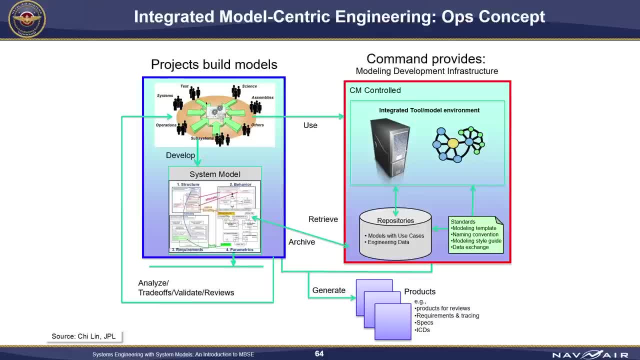 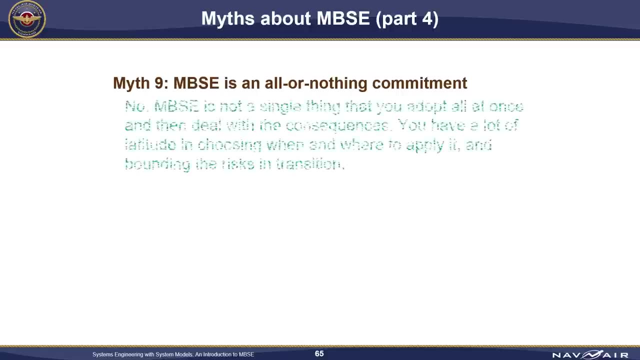 it is possible to generate various types of engineering products the projects need, but using the command-provided tools. that would be the same for all projects. Now let's look at one last myth: MBSE is an all-or-nothing commitment. No, 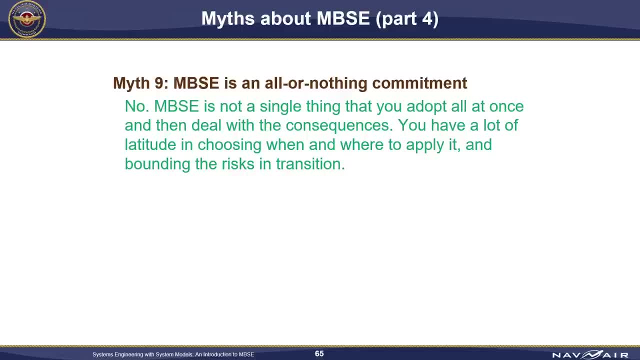 MBSE is not a single thing that you adopt all at once and then deal with the consequences. You have a lot of latitude in choosing when and where to apply it and bounding the risks in transition. MBSE involves a cultural change and it can progress step by step. 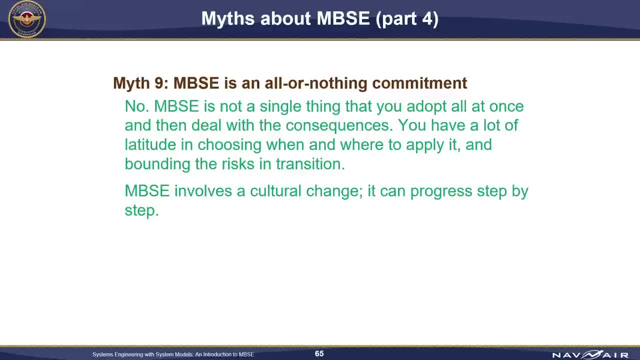 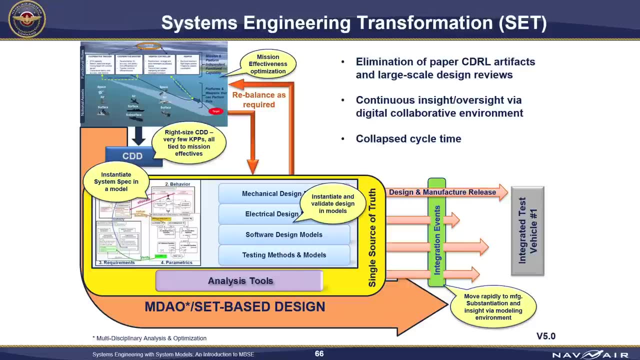 so you can take it a step at a time. This is the NAVAIR Systems Engineering Transformation Framework that was developed to describe the model-based systems engineering flow from the development of the mission-level requirements through the design and manufacture release. The intent of this framework. 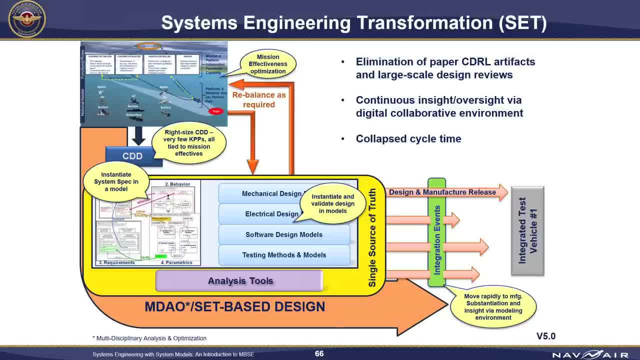 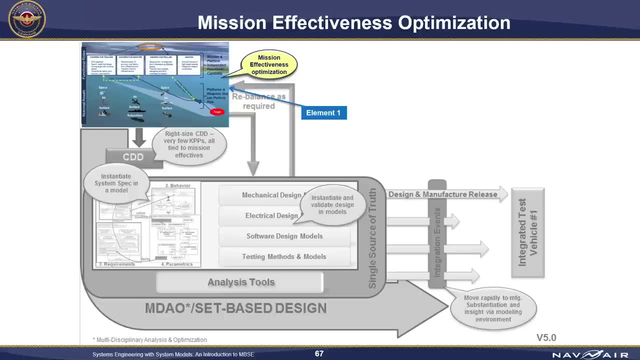 is to provide a digital thread through which we can apply optimization techniques and collapse the cycle time of the development efforts, as well as provide a system that meets the mission requirements. Element 1 of the framework comprises defining requirements at the mission level, including the mission-level architecture. 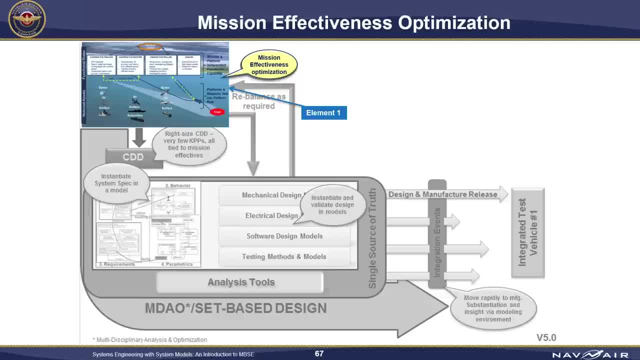 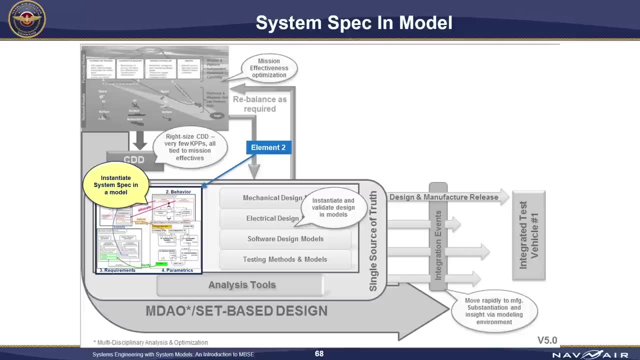 The requirements are right-sided and then flowed down to individual weapon systems, and may be rebalanced if necessary, based on the progression of the weapon system development. Element 2 is the instantiation of the system spec in a SysML model. By doing this, we capture and correlate.